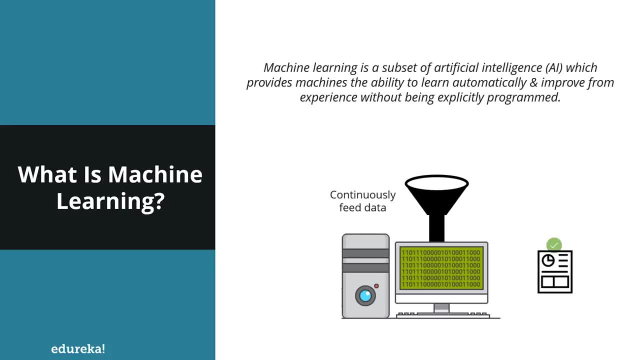 make more accurate predictions. Obviously, machine learning is not so simple. In order for a machine to analyze and get useful insights from data, it must process and study the data by running different algorithms on it. All right, And today we'll be discussing about. 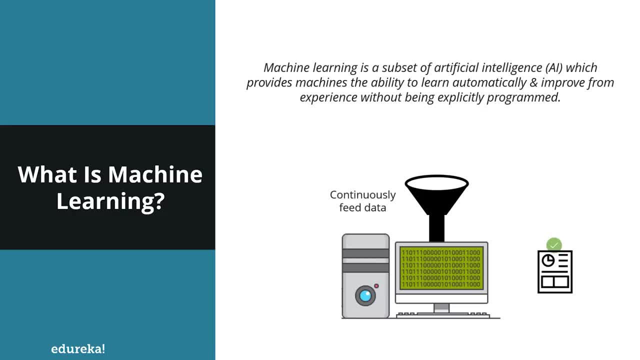 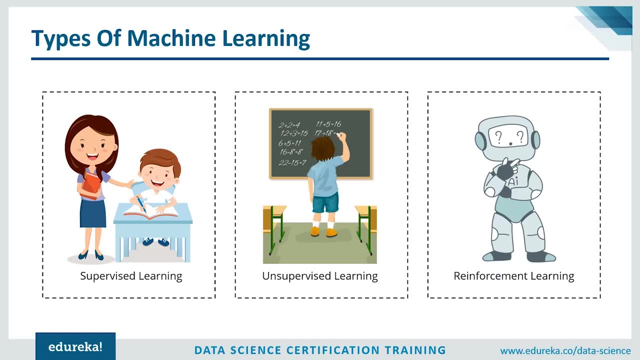 one of the most widely used algorithm called the support vector machine. Now that you have a brief idea about what machine learning is, let's look at the different ways in which machines learn. First, we have supervised learning In this type of learning. 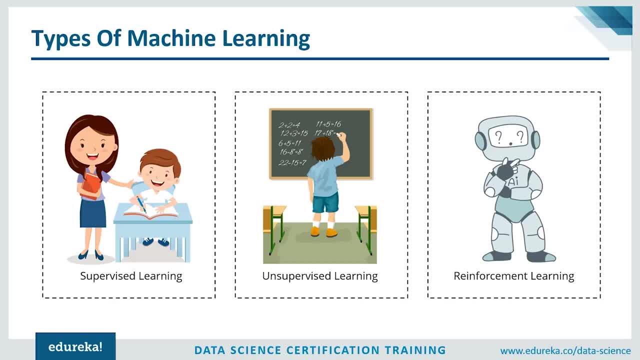 the machine learns under guidance. All right, That's why it's called supervised learning. Now, at school, our teachers guided us and taught us. Similarly, in supervised learning, machines learn by feeding them, label data and explicitly telling them: hey, this is. 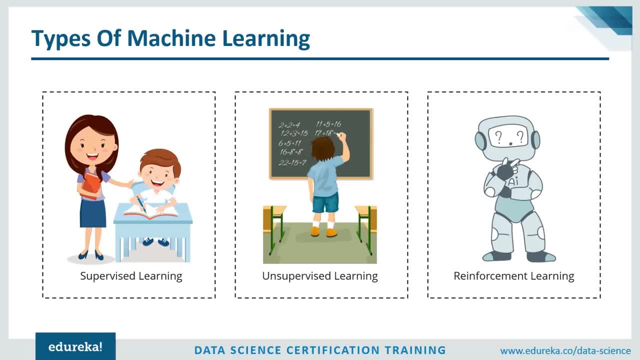 the input and this is how the output must look. Okay, So, guys, the teacher in this case is a training teacher. Next, we have unsupervised learning. Here, the data is not labeled and there is no guide of any sort. Okay, The machine must figure out the data set given and must find hidden. 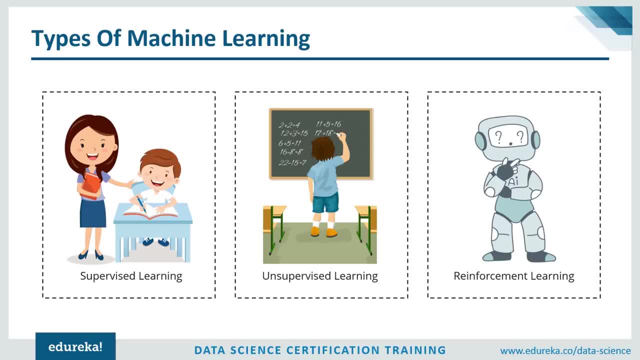 patterns in order to make predictions about the output. An example of unsupervised learning is an adult like you and me. We don't need a guide to help us with our daily activities. We figure things out on our own without any supervision. All right, That's exactly how. 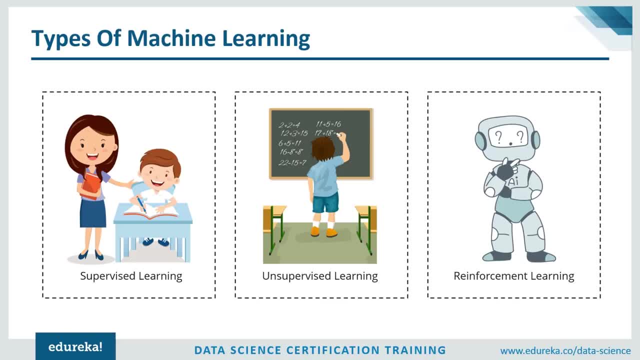 unsupervised learning works. Finally, we have reinforcement learning. Let's say you were dropped off at an isolated island. What would you do Now? initially you'd panic and you'd be unsure of what to do, where to get food from, how to live. 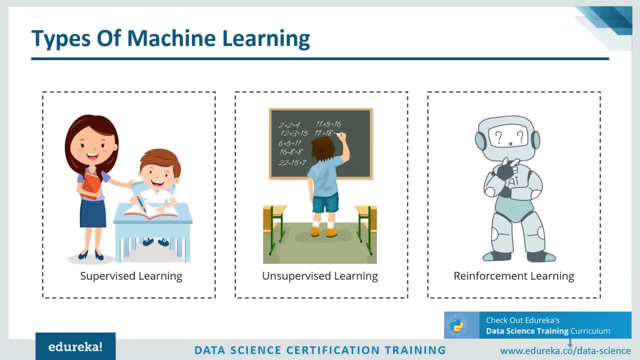 and all that, but after a while you will have to adapt. You must learn how to live in the island, adapt to the changing climate, learn what to eat and what not to eat. You're basically following the hit-and-drial concept because you're new to the surrounding and 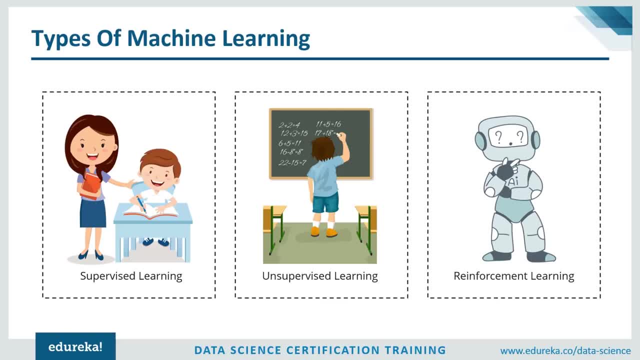 the only way to learn is experience, And then learn from your experience. This is exactly what reinforcement learning is Now, in real life. you will be alone, You will have to. learning is: It is a learning method wherein an agent interacts with its environment by producing. 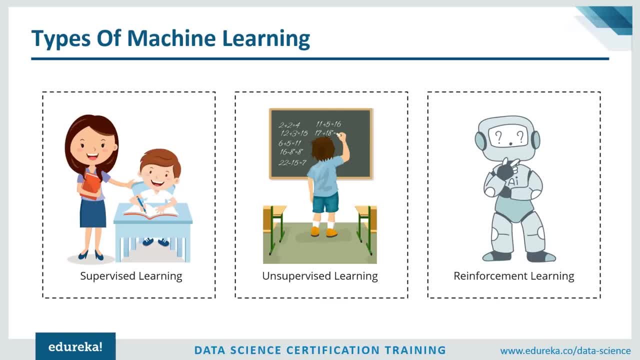 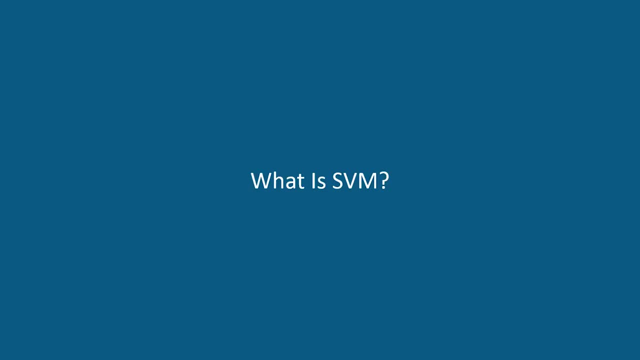 actions and discovers errors or rewards- Alright. and once it gets trained, it gets ready to predict the new data presented to it. Now, in our case, the agent was you, basically stuck on the island, and the environment was the island- Alright, okay, now let's move on and see what SVM algorithm is. 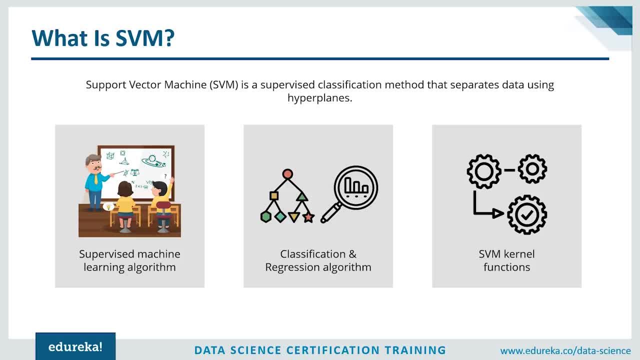 all about So guys? SVM, or support vector machine, is a supervised learning algorithm which is mainly used to classify data into different classes. Now, unlike most algorithms, SVM makes use of a hyperplane, which acts like a decision boundary between the various classes. In general, SVM can 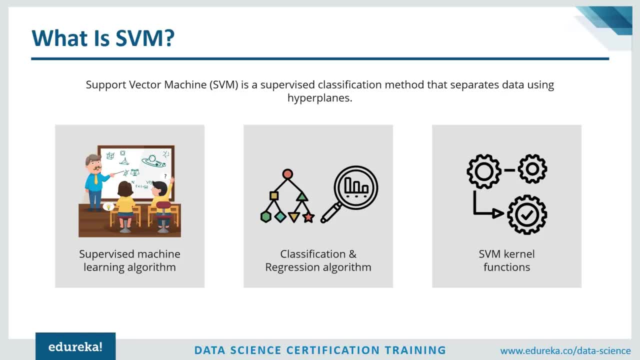 be used to generate multiple separating hyperplanes so that the data is divided into segments. Okay, and each of these segments will contain only one kind of data. It's mainly used for classification purpose, wherein you want to classify a data into two different segments depending on the features of the data. Now, before moving any further, let's 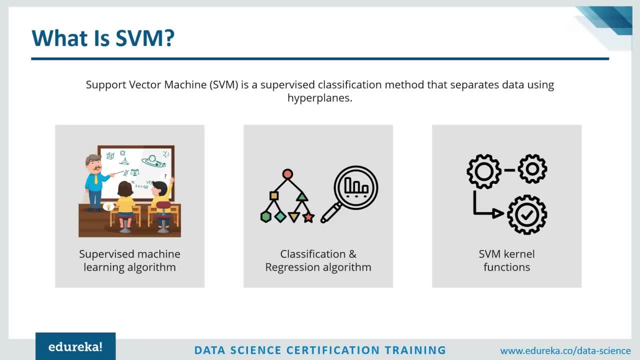 discuss a few features of SVM. Like I mentioned earlier, SVM is a supervised learning algorithm. This means that SVM trains on a set of label data. SVM studies the label training data and then classifies any new input data depending on what it learned in the training phase. A main advantage of 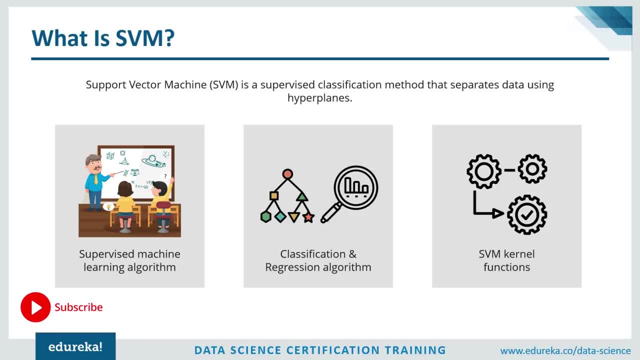 support vector machine is that it can be used to classify data into two different segments. SVM is mainly used for classification and regression problems. Now, even though SVM is mainly known for classification, the SVR, which is the support vector regressor, is used for regression problems. So SVM 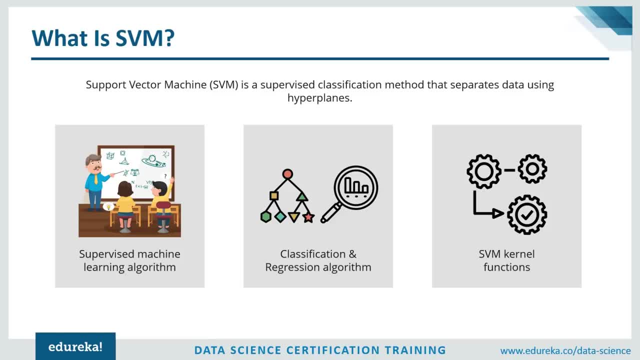 can be used both for classification and for regression. Now, this is one of the reasons why a lot of people prefer SVM, because it's a very good classifier and, along with that, it is also used for regression. Okay, another feature is the SVM kernel. So SVM is a very good classifier and 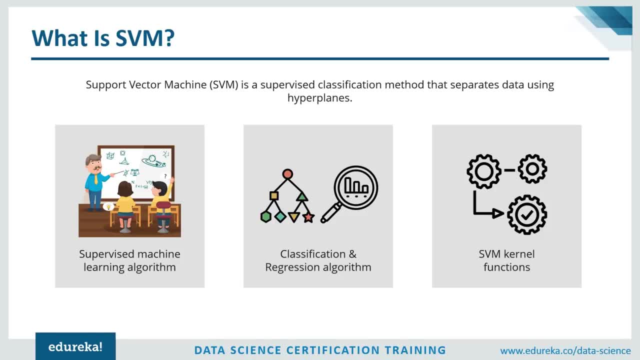 regression function SVM can be used for classifying non-linear data by using the kernel trick. The kernel trick basically means to transform your data into another dimension so that you can easily draw a hyperplane between the different classes of the data. All right, non-linear data is. 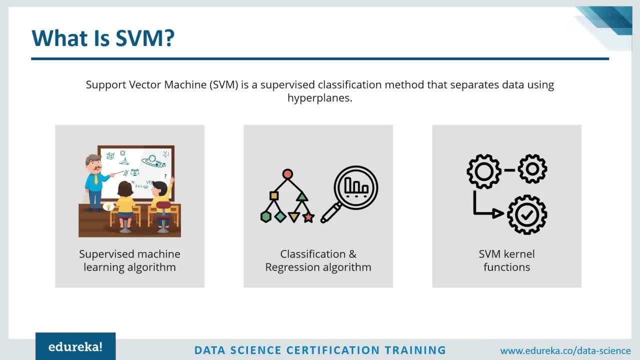 basically data which cannot be separated with a straight line. All right, so SVM can even be used on non-linear data sets. You just have to use the kernel functions to do this. All right. so, guys, I hope you all are clear with the basic concept. 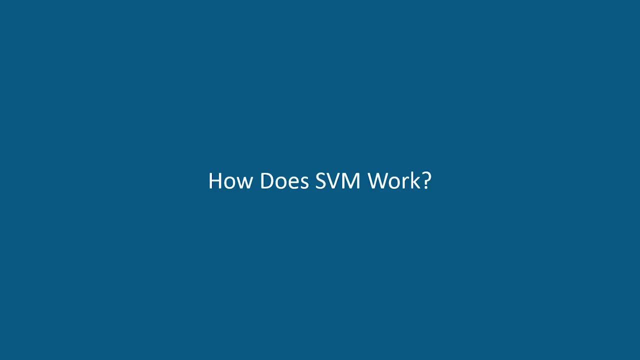 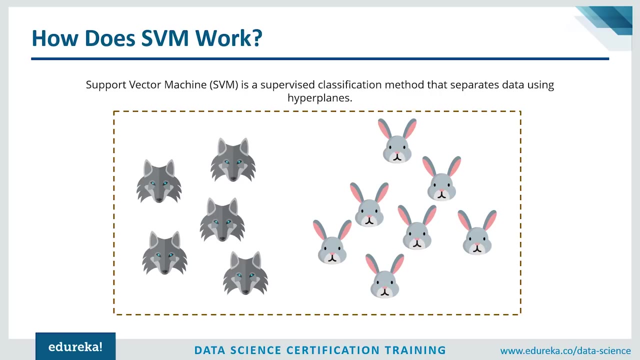 of SVM. Now let's move on and look at how SVM works. So, guys, in order to understand how SVM works, let's consider a small scenario Now for a second. pretend that you own a farm, Okay, and let's say that you have a problem and you want to set up a fence to protect your rabbits from the pack of. 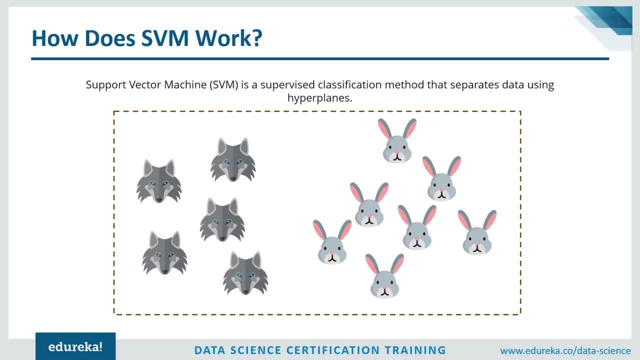 wolves. Okay, but where do you build your fence? One way to get around the problem is to build a classifier based on the position of the rabbits and wolves in your pasture. So what I'm telling you is: you can build a classifier based on the position of the rabbits and wolves in your pasture. 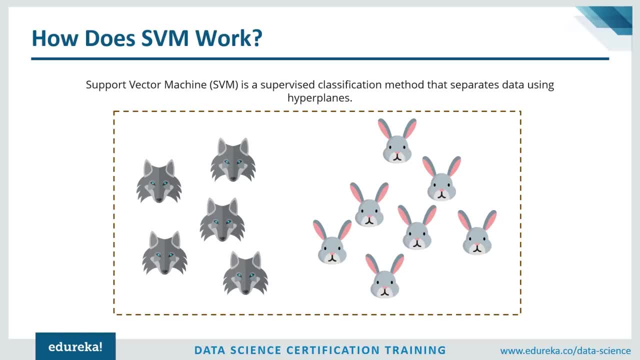 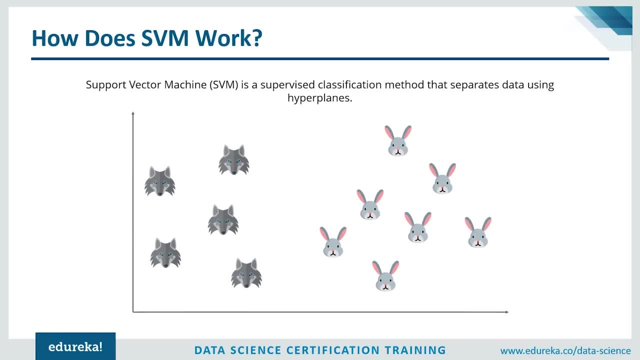 You can classify the group of rabbits as one group and draw a decision boundary between the rabbits and the wolves. All right, so if I do that and if I try to draw a decision boundary between the rabbits and the wolves, it looks something like this: Okay, now you can clearly build a fence along this line. 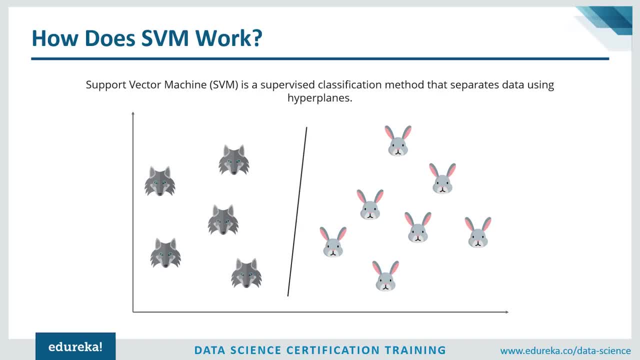 In simple terms, this is exactly how SVM works. It draws a decision boundary, which is a hyperplane, between any two classes in order to separate them or classify them. Now I know you're thinking: how do you know where to draw a hyperplane? The basic principle behind SVM is to draw a hyperplane. that 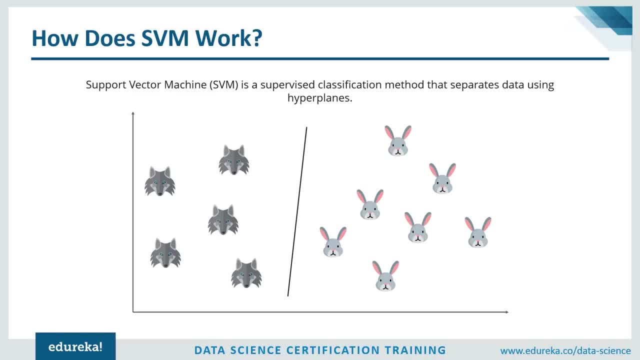 best separates the two classes. In our case, the two classes are the rabbits and the wolves. So you start off by drawing a random hyperplane and then you check the distance between the hyperplane and the closest data points from each class. These closest or nearest data points to the 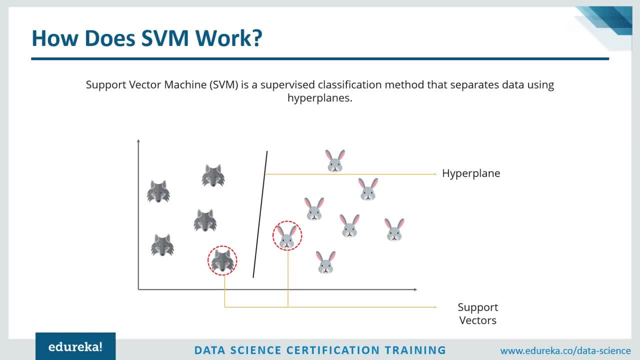 hyperplane are known as support vectors, and that's where the name comes from: support vector machine. So, guys, an optimum hyperplane will have a maximum distance from each of these support vectors. All right, so basically, the hyperplane which has the maximum distance from the support vectors. 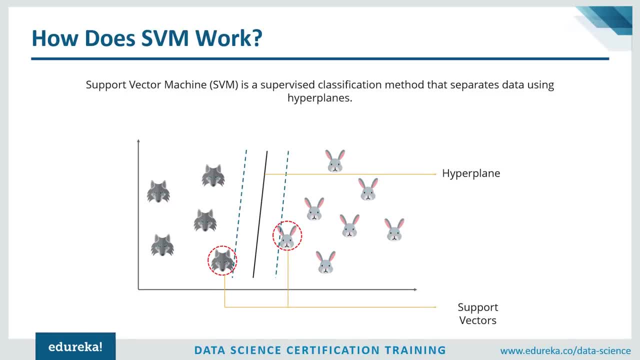 is the most optimum hyperplane, and this distance between the hyperplane and the support vectors is known as the margin. All right, so to sum it up, SVM is used to classify data by using a hyperplane, such that the distance between the hyperplane and the support vectors 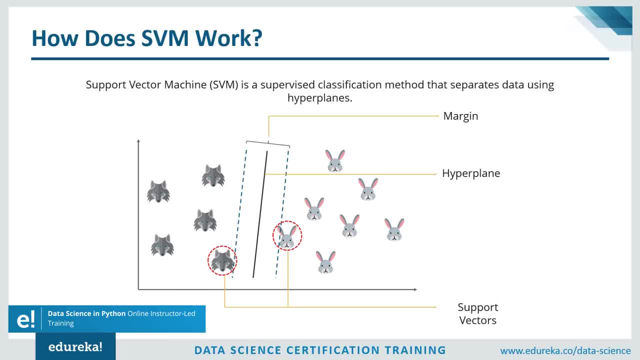 is maximum. So basically, your margin has to be maximum. All right, that way you know that you're actually separating your classes. All right, because the distance between the two classes is maximum. Okay, now let's try to solve a problem. Okay, so let's say that I input a new data point. Okay, this: 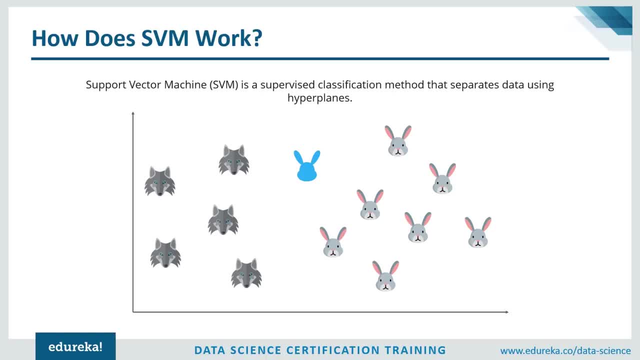 is a new data point and now I want to draw a hyperplane such that it best separates the two classes. Okay, so I start off by drawing a hyperplane like this and then I check the distance between the hyperplane and the support vectors. So I'm trying to check if the margin is maximum for this hyperplane. but what if I draw a hyperplane? 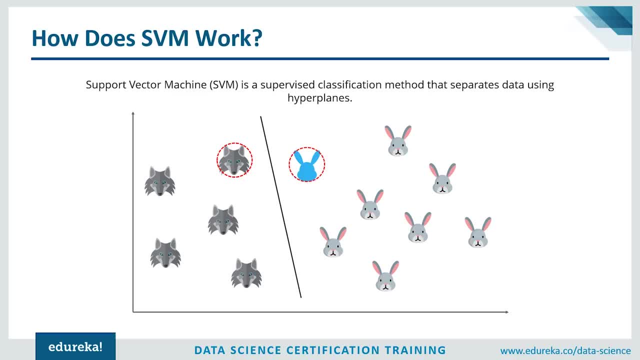 which is like this: All right, now I'm going to check the support vectors over here, Then I'm going to check the distance from the support vectors and for this hyperplane it's clear that the margin is more All right when you compare the margin of the previous one to 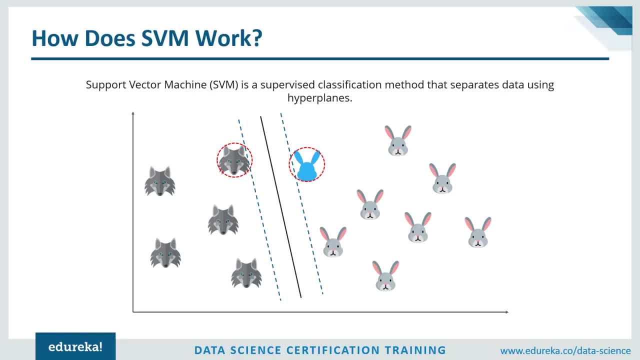 this hyperplane. it is more. So the reason why I'm choosing this hyperplane is because the distance between the support vectors and the hyperplane is maximum in this scenario. Okay, so, guys, this is how you choose a hyperplane. You basically have to make sure that the hyperplane 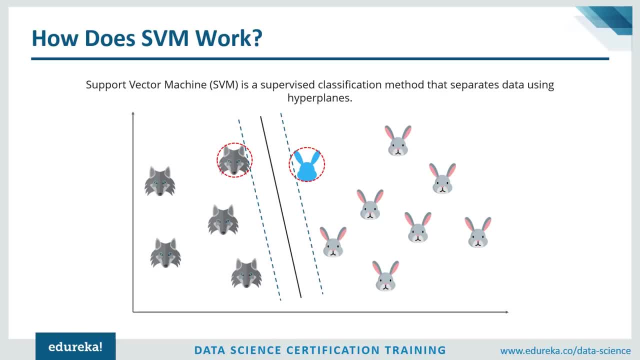 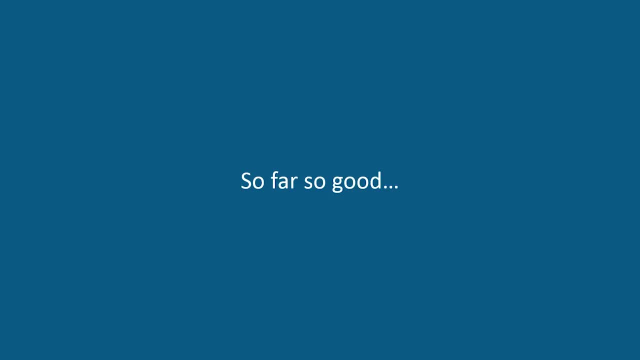 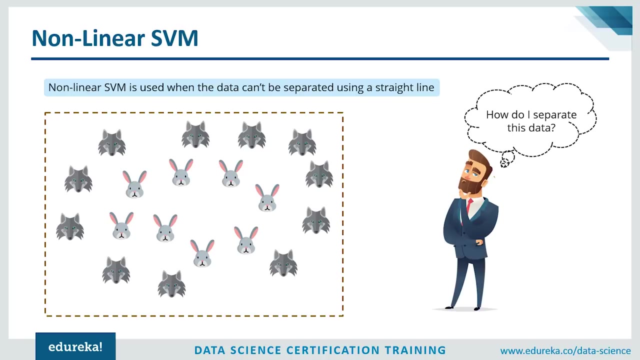 has a maximum margin, All right. it has to best separate the two classes, All right, okay, so far it was quite easy. Our data was linearly separable, which means that you could draw a straight line to separate the two classes. All right. but what will you do if the data set is like this? You possibly 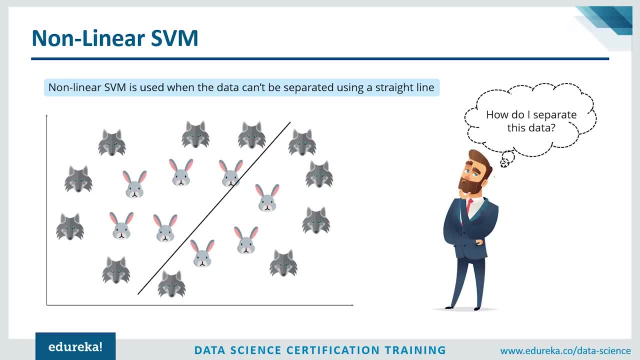 can't draw a hyperplane like this. All right, it doesn't separate the two classes at all. So what will you do if the data set is like this? You can't separate the two classes at all. So what you're going to do is you're going to use the kernel function to separate the two classes. All right, 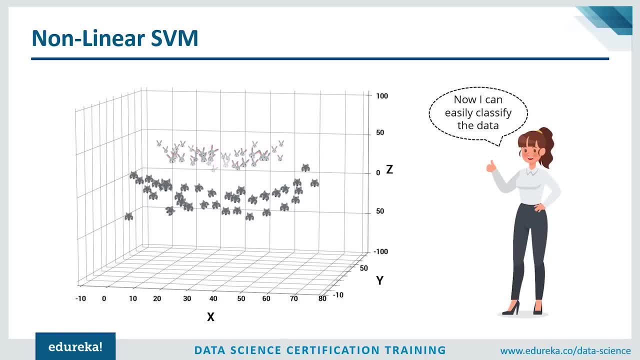 so the kernel function is going to be used to separate the two classes at the same time. All right. so kernel functions offer the user this option of transforming non-linear spaces into linear ones. Non-linear data set is the one that you can't separate using a straight line. All right, 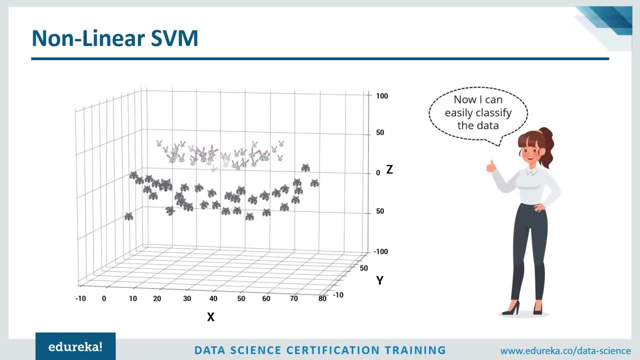 in order to deal with such data sets. you're going to transform them into linear data sets and then use SVM on them. Okay, so a simple trick would be to transform the two variables x and y into a new feature space involving a new variable called z. All right, so, guys, so far we were plotting our 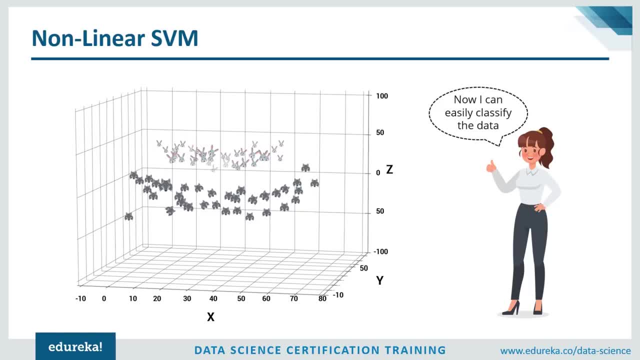 data on two dimensional space. Correct, we were only using the x and the y axis, So we had only those two variables, x and y. Now, in order to deal with this kind of data, a simple trick would be to transform the two variables x and y into a new feature space. 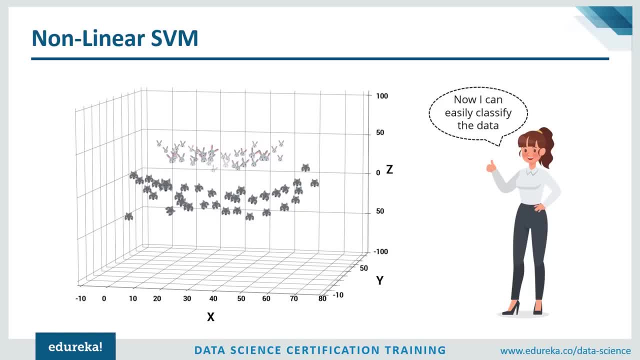 involving a new variable called z. Okay, so we're basically visualizing the data on a three dimensional space. Now, when you transform the 2d space into a 3d space, you can clearly see a dividing margin between the two classes of data. All right, now you can go ahead and separate the. 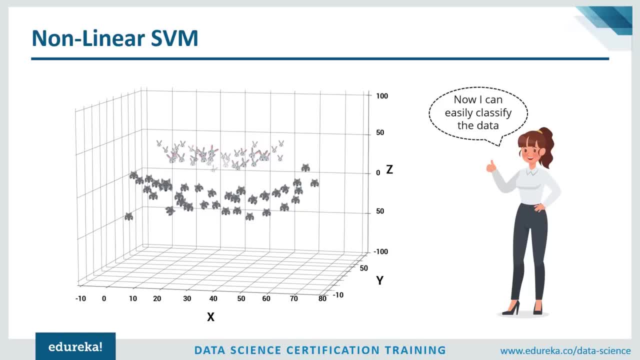 two classes by drawing the best hyperplane between them. Okay, that's exactly what we discussed in the previous slides. So, guys, why don't you try this yourself? try drawing a hyperplane which is the most optimum for these two classes. All right? so, guys, I hope. 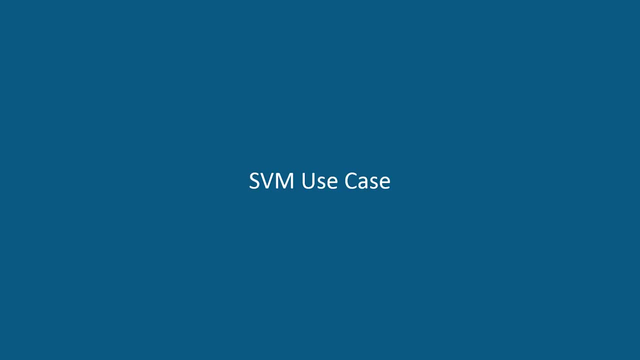 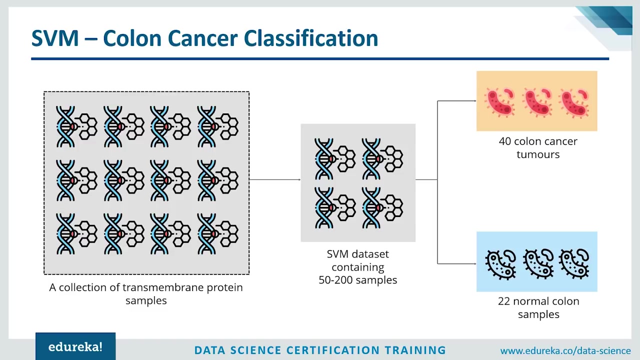 you have a good understanding about non-linear SVMs. Now let's look at a real world use case of support vector machines. So, guys, SVM as a classifier has been used in cancer classification since the early 2000s. So there was an experiment held by a group of professionals who applied SVM. 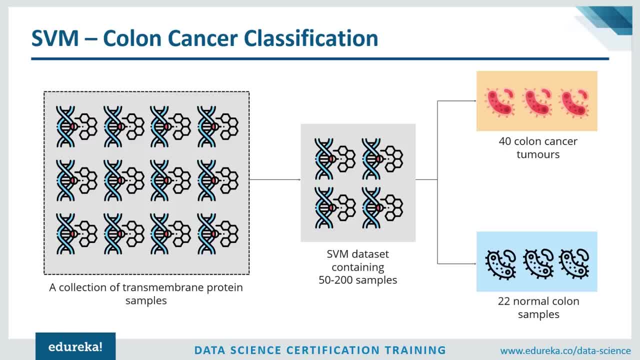 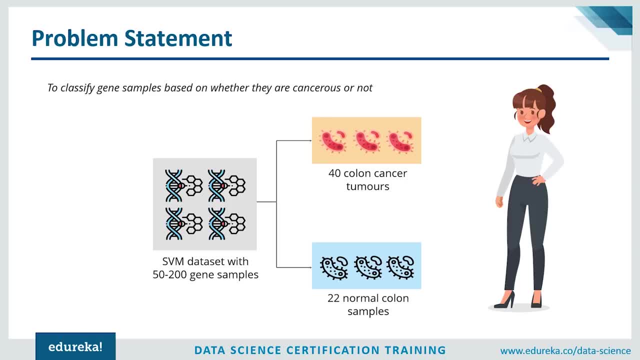 in a colon cancer tissue classification. So the data set consisted of about 2000 transmembrane protein samples and only about 50 to 200 gene samples. These samples were input into the SVM classifier. Now, this sample which was input into the SVM, 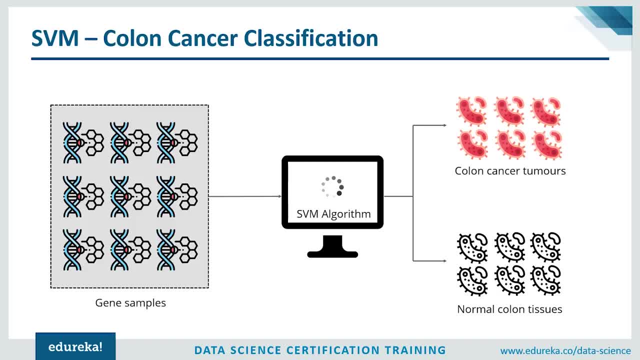 classifier had both colon cancer tissue samples and normal colon tissue samples. All right now. the main objective of the study was to classify gene samples based on whether they are cancerous or not. Okay, so SVM was trained using the 50 to 200 samples in order to discriminate between 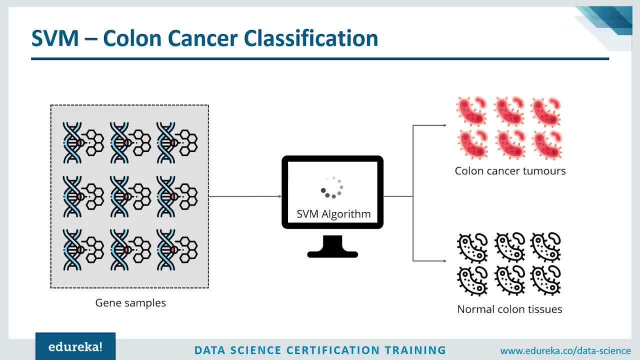 non-tumor from tumor specimens. So the performance of the SVM classifier was very good for even a small data set. All right, we had only 50 to 200 samples and even for the small data set, SVM was pretty accurate with its results. Not only that, its performance was compared to. 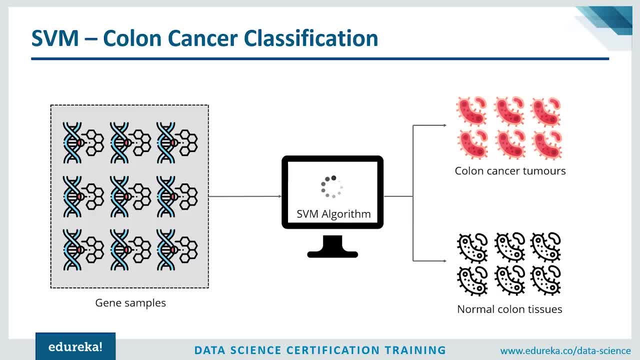 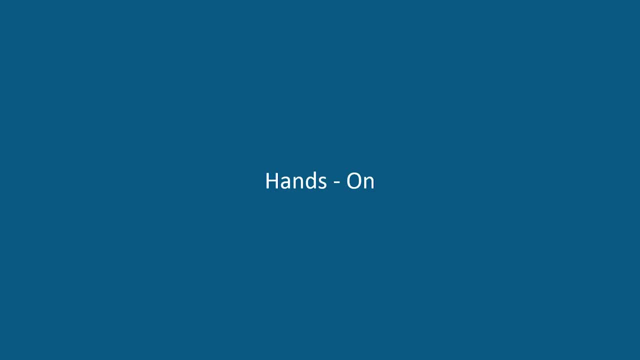 other classification algorithms like naive Bayes, and in each case SVM outperformed naive Bayes. So after this experiment, it was clear that SVM classified the data more effectively and it worked exceptionally good with small data sets. All right, now let's get into the practical part. We'll run a 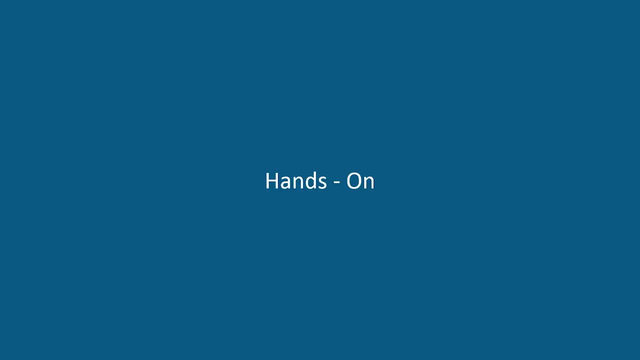 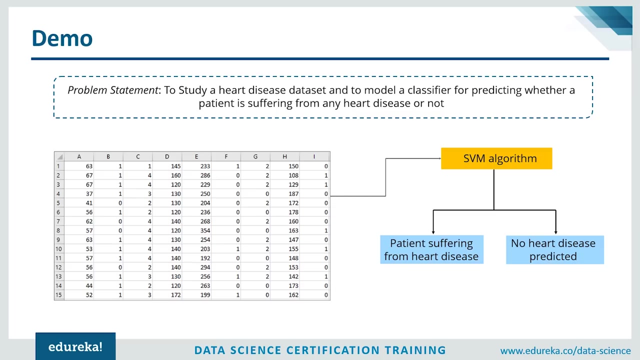 little bit of a demo to better understand how SVM can be used as a classifier. Okay, so, guys, before we run the demo, let's look at our problem statement. So our problem statement is to study a heart disease data set and build a classifier to predict whether a patient is suffering from heart disease. 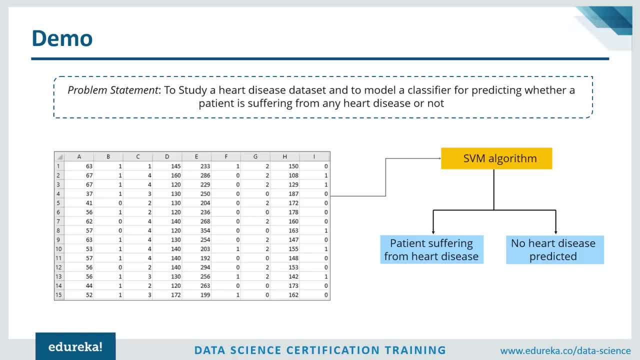 or not. All right now. this data set will have n number of patients, along with details about the patients, Okay, for example, their age, the cholesterol level, their sex- all that will be mentioned in the data set. Build a SVM classifier and then predict whether a patient is suffering from any heart disease or not. 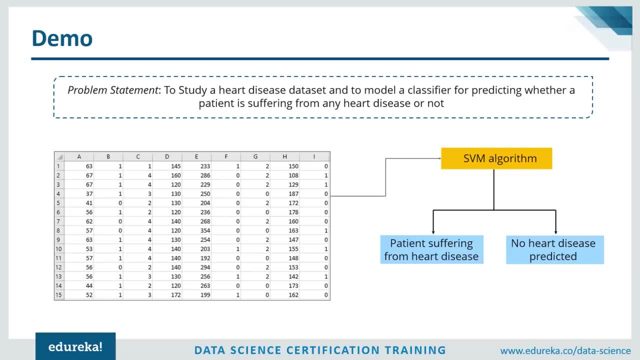 All right, so we're creating two classes over here. One class consists of patients suffering from heart disease and the other class is the lucky one which is not suffering from any sort of heart disease. All right, so let's move on and look at today's demo. So, guys, in order to save some time, I've already 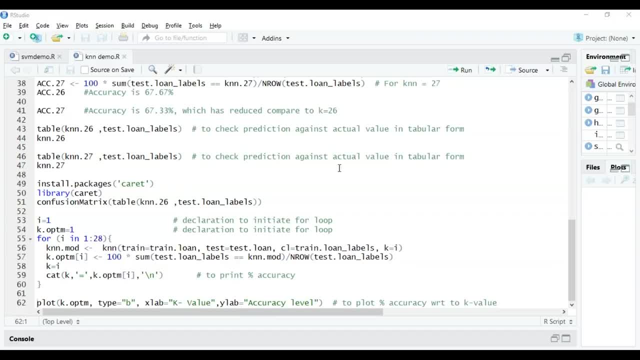 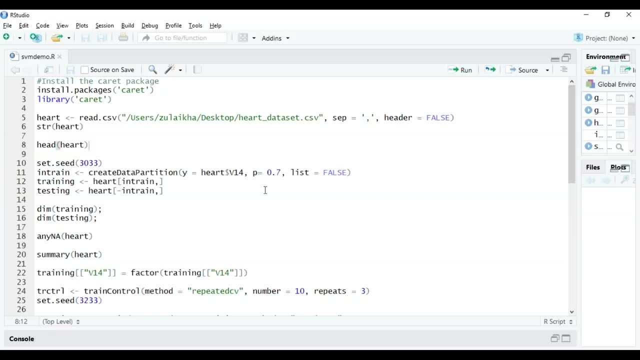 typed out the code, but don't worry, I'm going to explain each and every line of code over here. All right, now, guys, in our demo, we'll be using the carrot package. all right, the carrot package, which is also known as a classification and regression training. it has tons of functions which 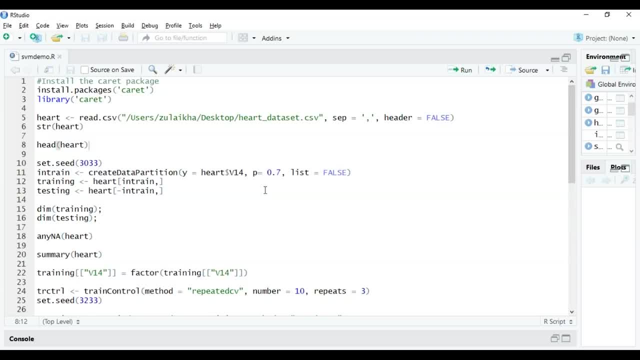 can help us to build predictive models. so it contains tools for data splitting, pre-processing, feature selection tuning, supervised and unsupervised learning algorithm. okay, so to use it, we first need to install it using this command: install dot packages- carrot- alright, the carrot package is very helpful because 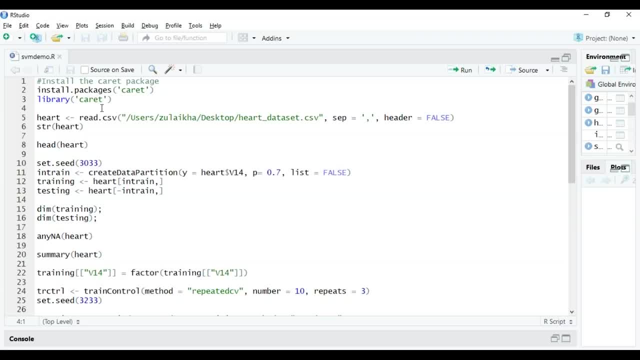 it provides us direct access to various functions. so for training our model, we require algorithms like en and SVM, decision tree, linear regression. all of these algorithms are already pre coded in the carrot package. okay, so after installing it, we just need to load the package into our console. to do that, we 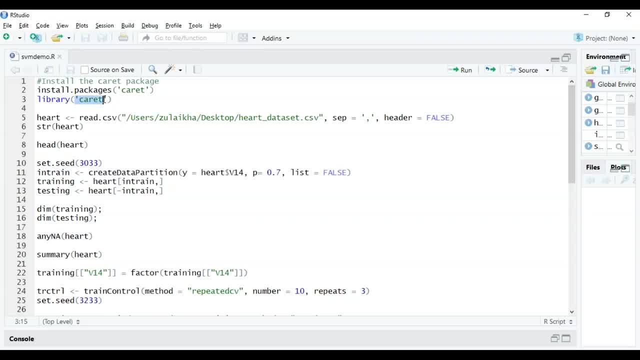 have this code snippet, which is library and the name of the package. okay, so our next step is to load the data set. so, guys, for this demo, we'll be using a heart disease data set which consists of a code snippet, which is a code snippet which is a function called DARPA 35, and the data set is a data set which consists: 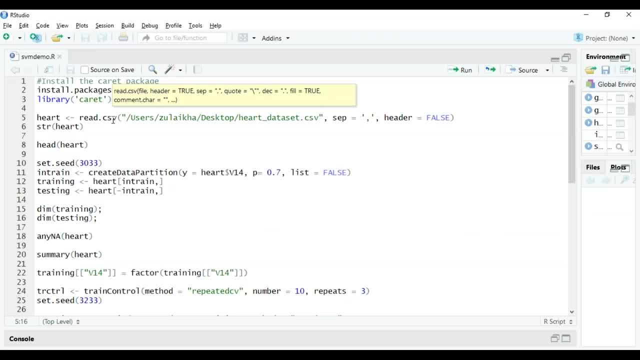 of various attributes, like the person's age, sex, cholesterol level and etc. in the same data set, we have a target variable which is used to predict whether a patient is suffering from any heart disease or not. okay, I'll show you the target variable in a bit. okay, so this is the aim of our demo they're going to use. 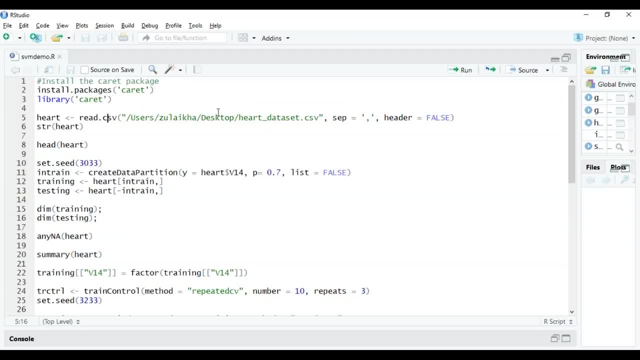 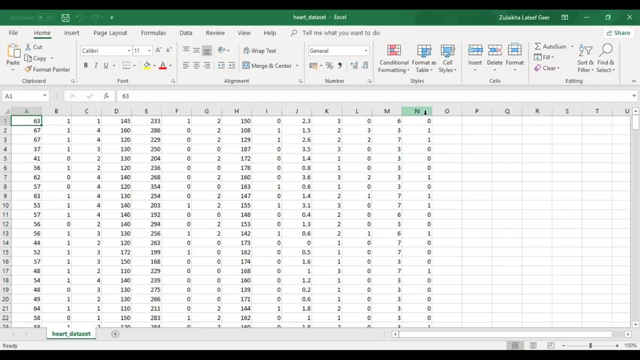 the SVM to classify whether a person is going to be prone to a heart disease or that. let me just show you the data set So you can see that it has around 14 attributes. okay, till column n and the last attribute over here. 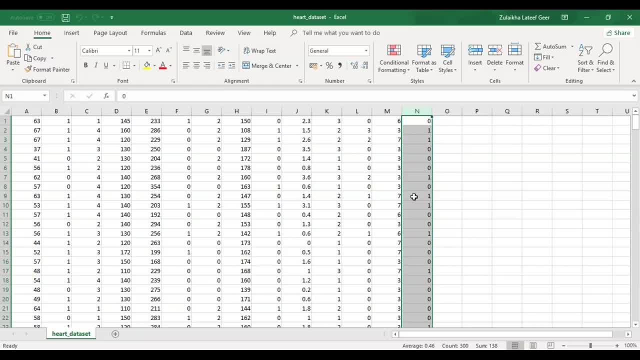 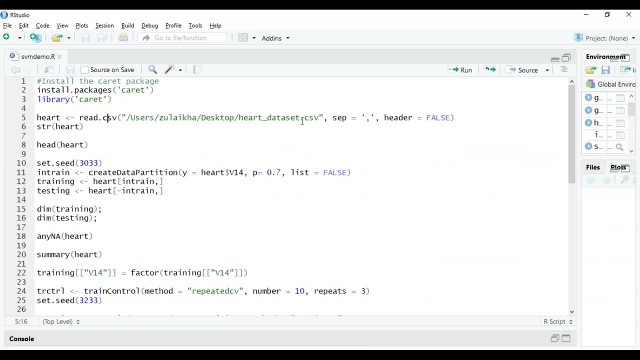 the n column is the target variable. Okay, we'll be predicting this using our SVM model. Okay, so, guys, I already have the data set. Now all I have to do is I need R to read the data set from my machine. okay, 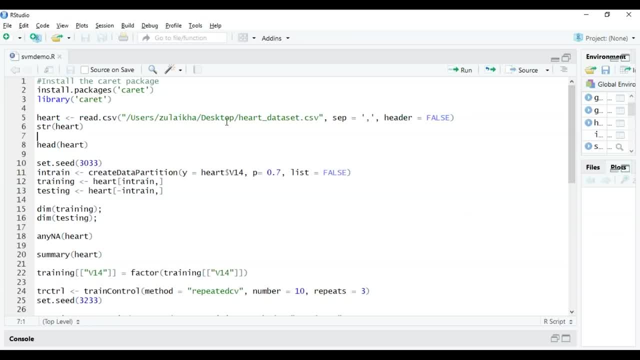 So to do that, we have this line of code. So what I'm doing here is: this is the name of my data set: heart underscore. data set: dot CSV. Okay, it's stored in a CSV or a comma separated file. All right, now the location of this data set is over here. 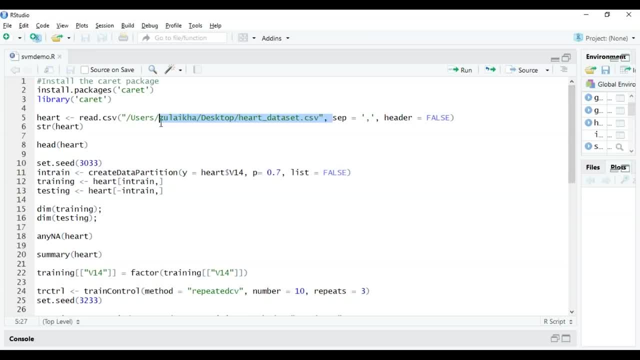 users: lakehard desktop. Okay, this is basically the path to my data set. After that, there is another field called separator. Okay, this just identifies that this is a comma separated file. And lastly, we have another parameter which says header. 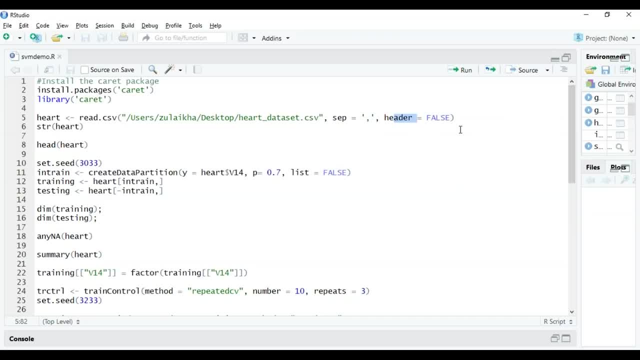 Header indicates whether my data set has a header or not. Okay, in this case it's false, all right, So, guys, I'm basically using this readcsv function to read my data set, all right, And I'm storing the data set in a variable called heart. 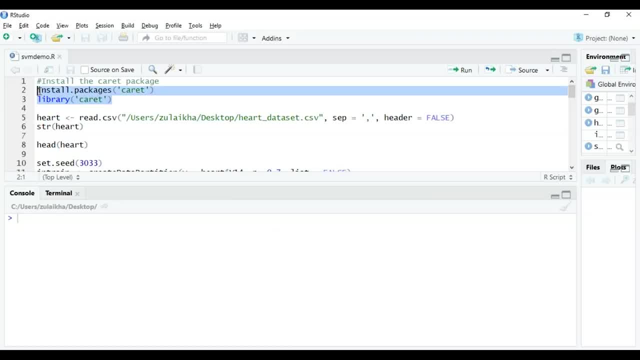 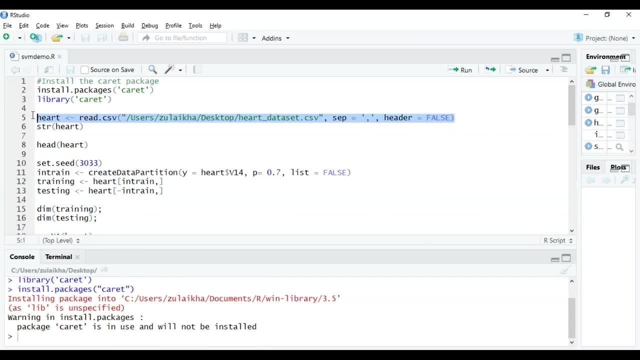 Now let's run this line of code. Run both of these lines first. Okay, Now let me run this line of code. Okay, all right, now that we've imported our data set, let's check the structure of our data set. okay. 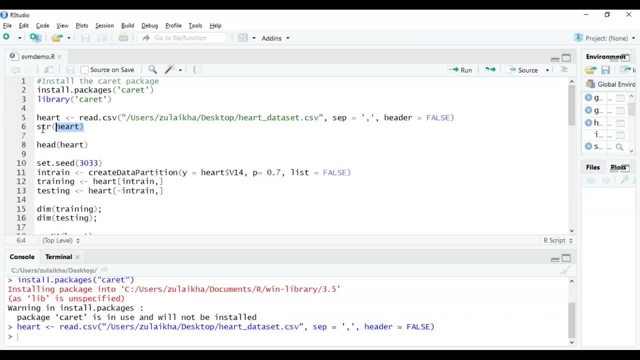 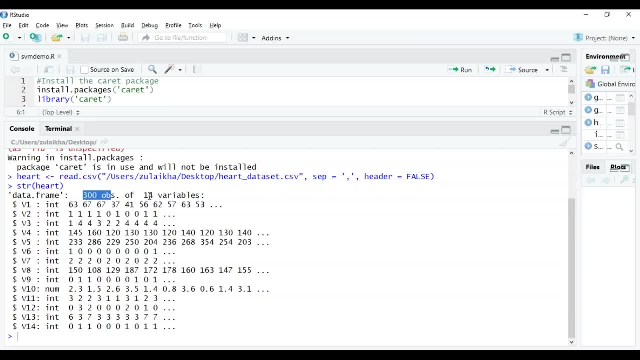 So you use this function called str to check the structure of your data set. So it basically has 14 attributes and it shows us that there are 300 observations and 14 variables over here. okay, So, guys, all of these values are converted. 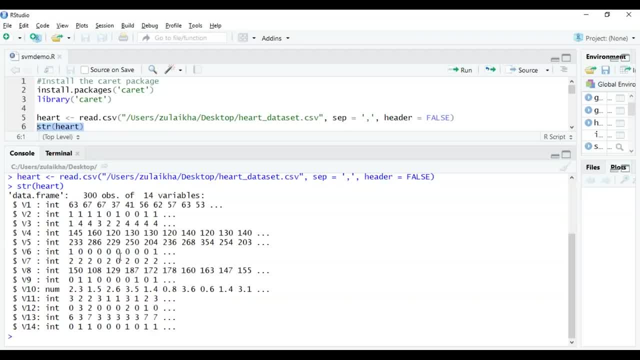 into numerical format. So that's why you might not be able to understand this data set. But in order for R to run this data set, it has to be in numerical form. For this to perform any computation on the data set, it has to be in numeric form. all right. 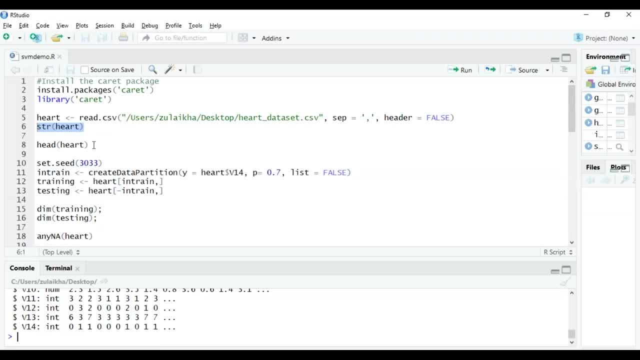 Okay, then, if you want to display the first five, six rows of your data set, you can use the head function. All right, this head function will display the first five, six observations of your data set. all right, So this is what our data set looks like. 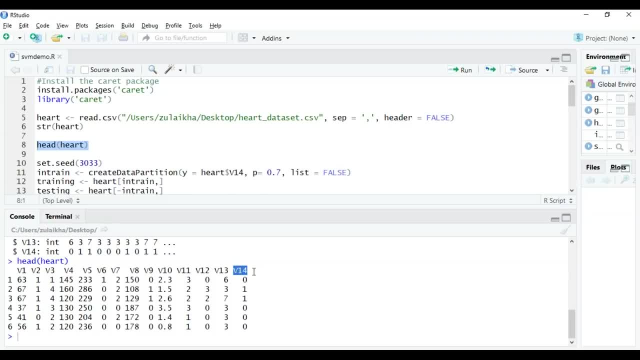 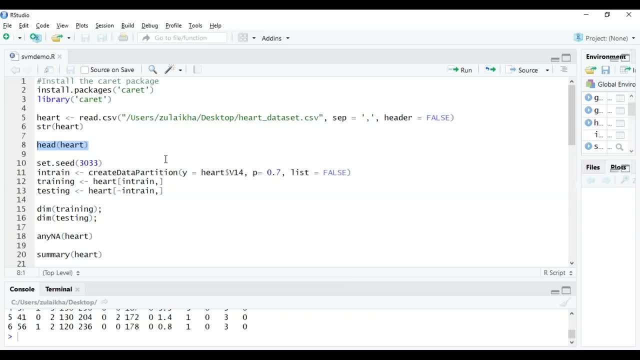 These are all the attributes. Okay, there are 14 attributes and this is our target variable that we're gonna predict. All right now. our next step is to split the data into training set and the testing set. Okay now, this process is also called as data splicing. 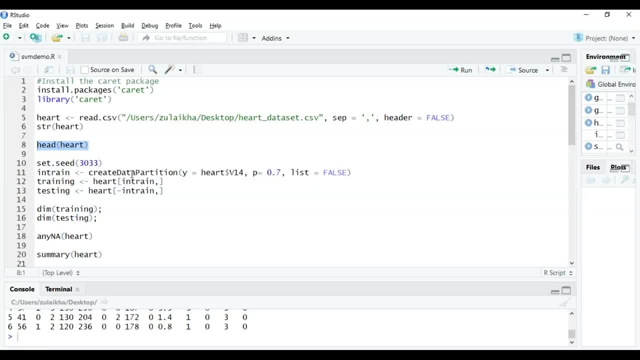 Okay, so we're going to use the training set specifically for our model building and the testing set for evaluating the model. all right, So this entire set of code is basically for splitting the data. okay, Now, here you can see this: create data partition function. 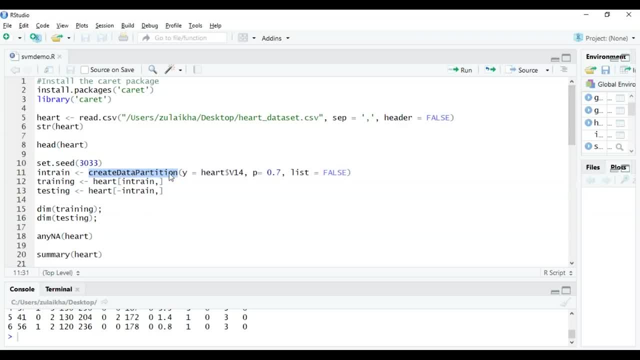 So the caret package provides a method called the create data partition, which is basically for partitioning our data into training and testing set. Okay, here you can see that to this function I've passed three parameters: y, p and list. 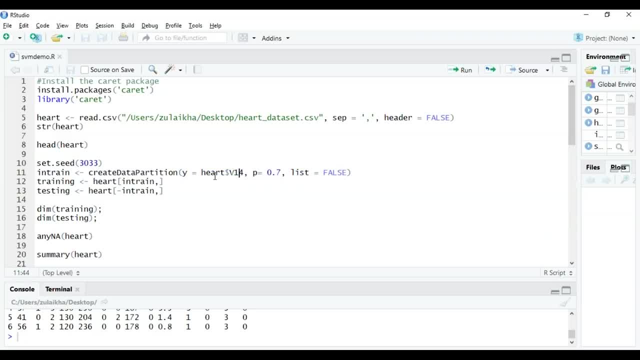 Now the y parameter takes the target variable into consideration. okay, So it checks that within my heart data set v14, which is my target variable. All right, our next parameter. p basically holds a decimal value. Now p basically stores a decimal value from zero to one. 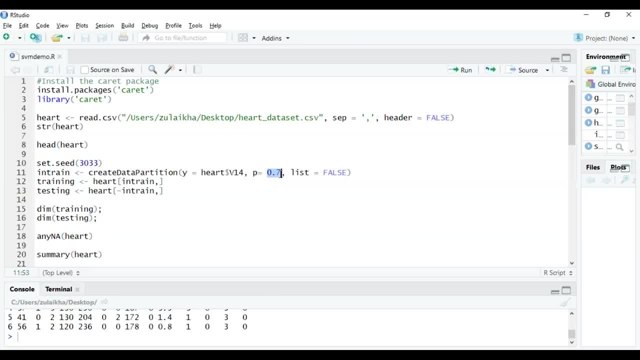 Okay, so between zero and one it has a value, and over here you can see that 0.7 is a value for p. It means that we're splitting our data in the ratio of 70 is to 30, okay. 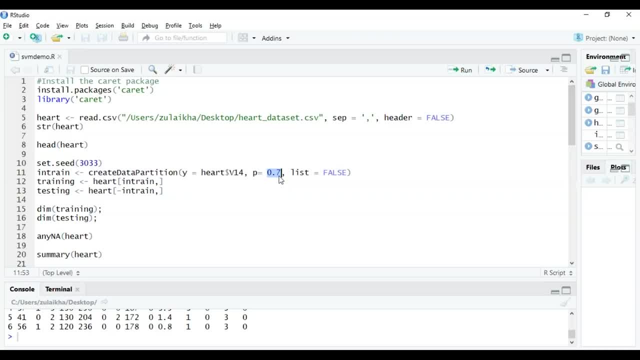 So 70% of our data is going to be used for testing- okay- For training- and the remaining 30% will be used for testing the model. okay, So I'm storing this in the intrain variable. okay, Then I'm assigning a new variable called training. 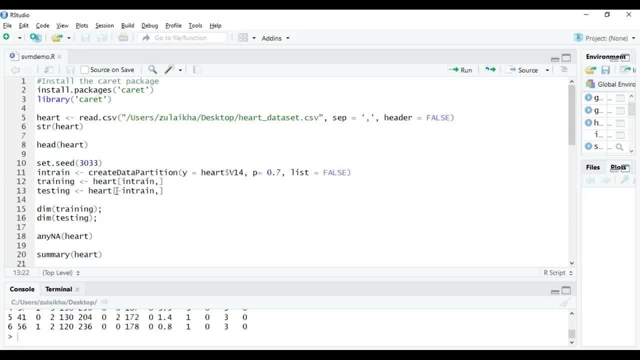 which contains my 70% of the data and the remaining. that's why it says minus intrain, which is the remaining data set, which is the 30% of the data is assigned to the testing variable. all right, So let's run the set of code. 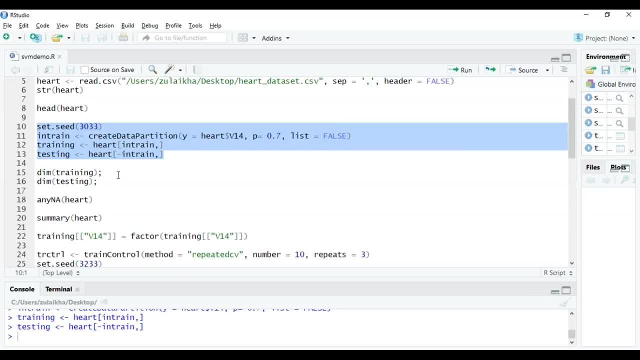 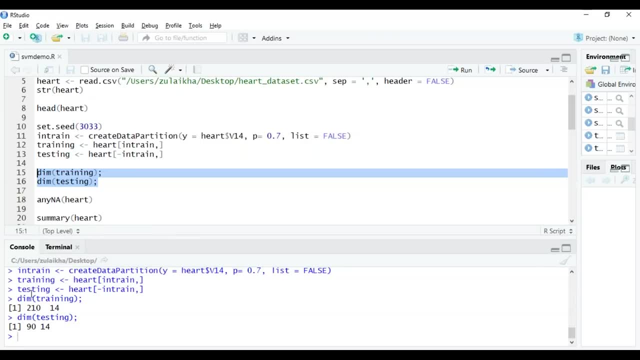 Next, for checking the dimensions of our training data frame and the testing data frame, we can use this dimension function. okay, DIM. Okay, let's look at the output. So the training data set has 210 observations with 14 variables, obviously 14 attributes. 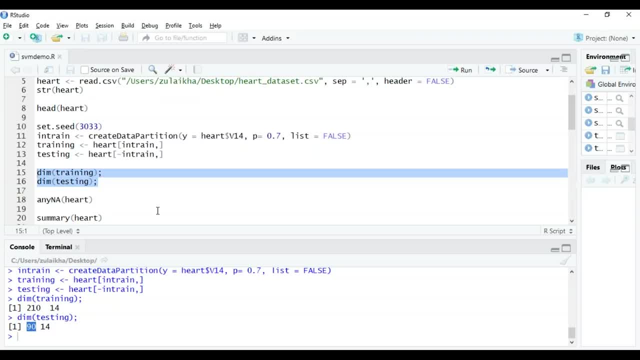 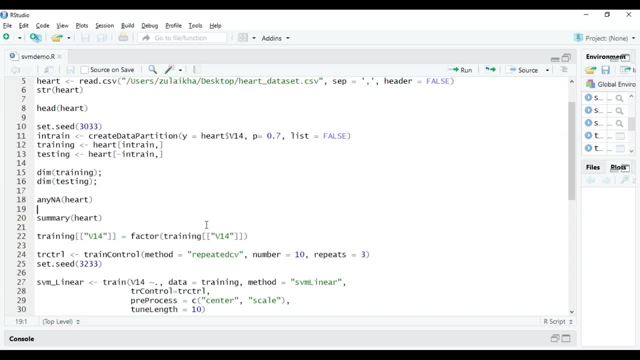 and 90 observations are present in the testing data set. All right, Okay, now our next step is to clean the data. So if there are any missing values or inconsistent values, they have to be dealt with before we build the training model. okay, 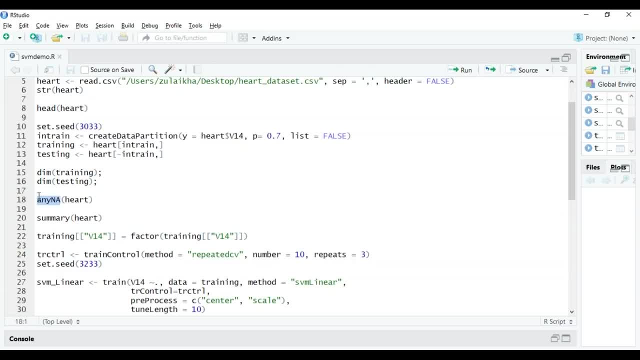 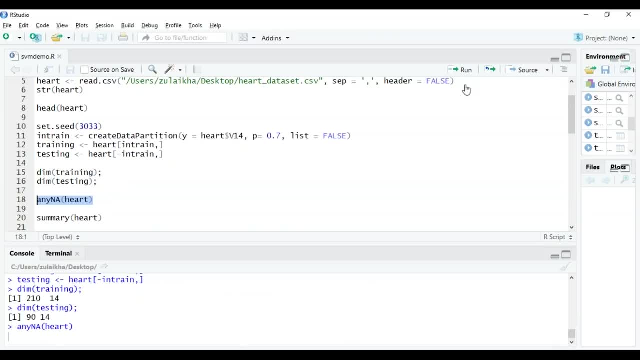 So here we're using the any any function, this function which checks for any null values or any non-available values. Okay, so let's run this. All right, on running this, we get the return value as false. Okay, here you can see that it says false. 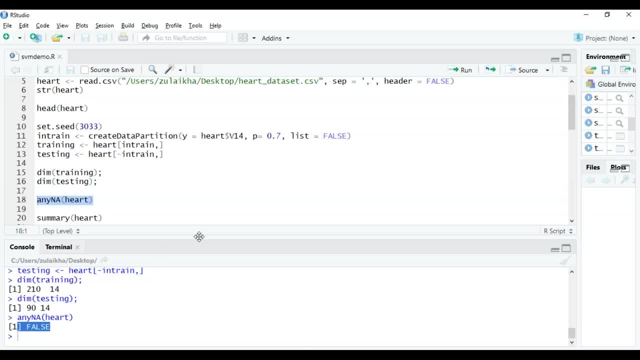 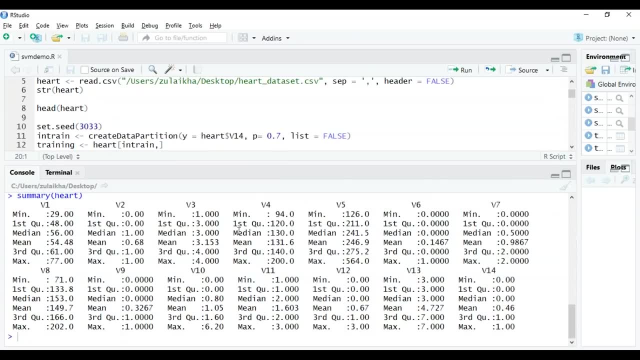 Okay, this means that there are no missing values in our data set and we're good to go All right. now let's finally check the summary of our data set to see if everything is correct. Okay, now. the output here shows that the values 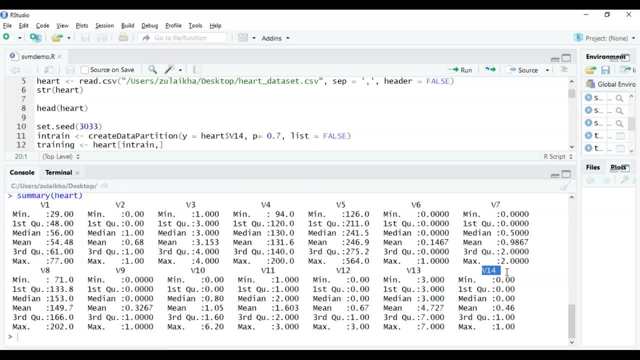 of various variables are not standardized. okay, will consider this v14 variable. okay, this is our target variable and it holds only two values: either it holds zero or it has one. okay, instead this should be a categorical variable. okay, to convert these two categorical variables we need. 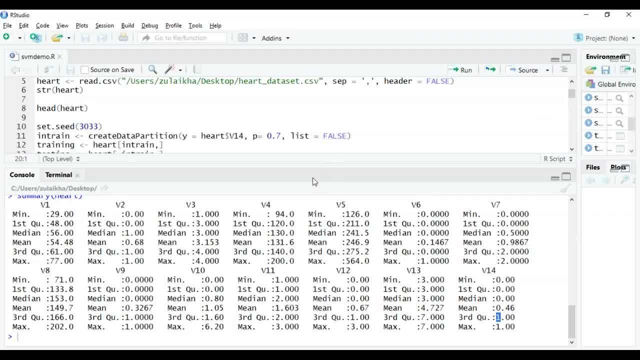 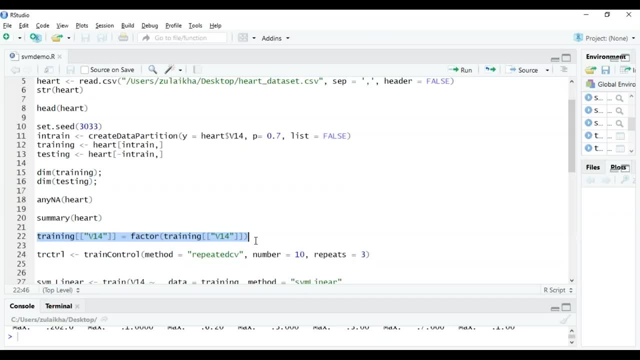 to factorize them. alright, so let's factorize the variable b14. okay, now this line over here. it basically converts a training data frame v14 column to a factor variable. okay, so this v14 variable. it will turn it into a factor variable. so let's run this on right now. our next step is to train our model. so 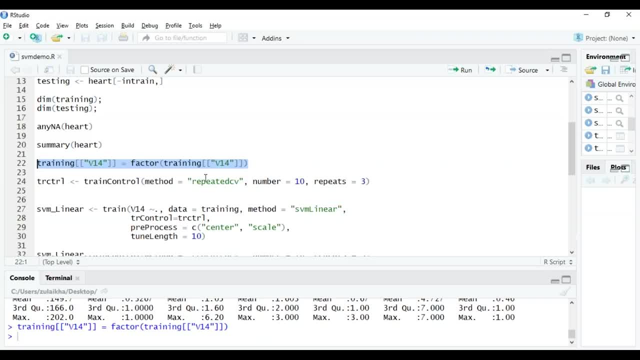 before we train our model, we will first implement the train control method. okay, here you can see the train control method. now this will control all the computational overheads so that we can use the train function provided by the carrot package. alright, here you can see in the next line, I've used the train. 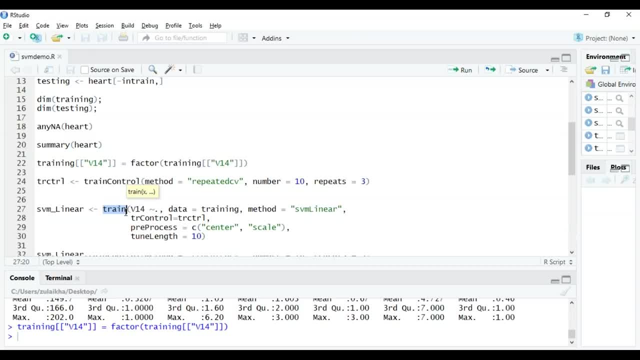 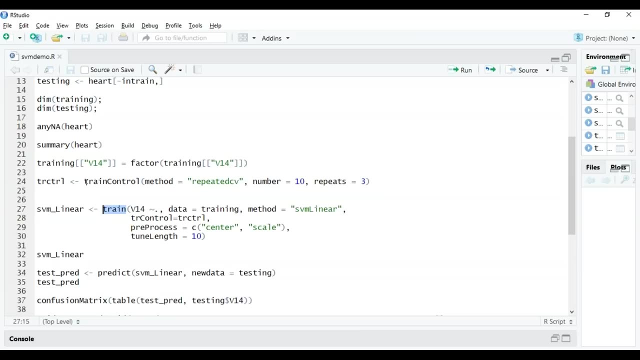 function. now, carriage package provides this function in order to train different algorithms. now, guys, this train method is offered by the carrot package itself. you can use it to train the data on different algorithms. okay, alright, so first let's focus on the train control method. okay, this method: train control. 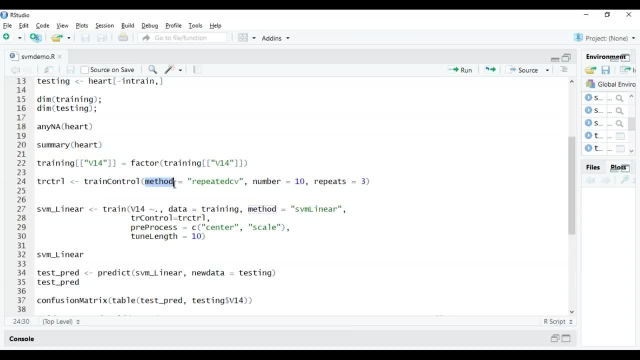 method here is taking three parameters. okay, it has a method attribute number and repeats. now the method parameter defines a resampling method and in this demonstration we exchange리 will be using the repeated CV or the repeated cross validation method. the next parameter is a number parameter. this basically holds a number of 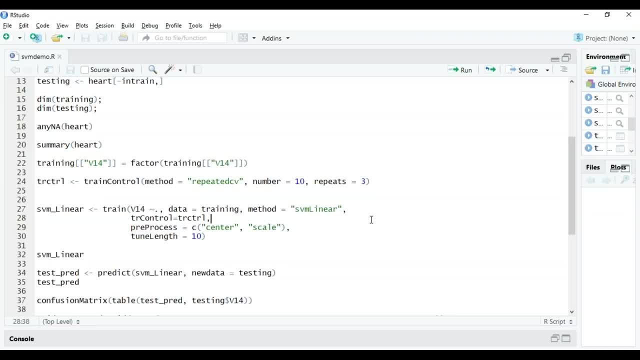 resampling iterations: okay, so how many iterations you want to do on this data set? and that is the number that this is going to represent? okay, the repeats parameter contains the sets to compute for a repeated cross validation. so here we're setting the number equal to 10 and the repeats equal to 3, all right, this. 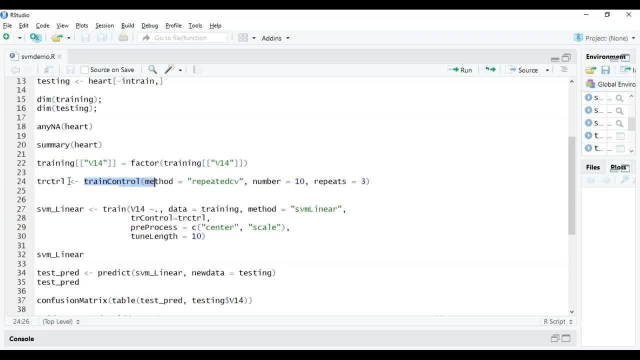 train control method will return a list to us on it which is basically going to be stored in this, and we're going to pass this to our training method. this is the train method. all right, so let's run this line of code. okay, so we've run that. 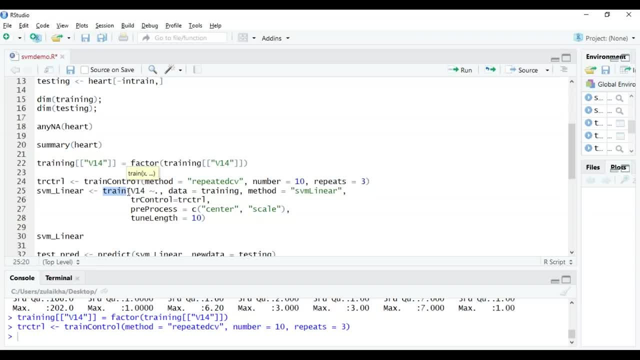 successfully. so now we have the train function. okay, now this function has to be passed with the method parameters set to SVM linear. okay, we are passing our target variable as well, which is B 14, and this dot and this ît approximation basically indicates that our model is using all the attributes in our classifier. 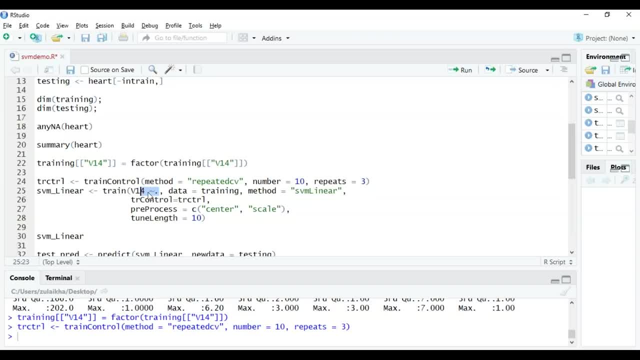 and v14 is a target variable. okay, it's indicating that v14 is our target variable and it's using all the attributes in the data set. next we have the tr control parameter. okay, this tr control parameter should be passed with the results from our train control method. okay, so, whatever, we ran in the 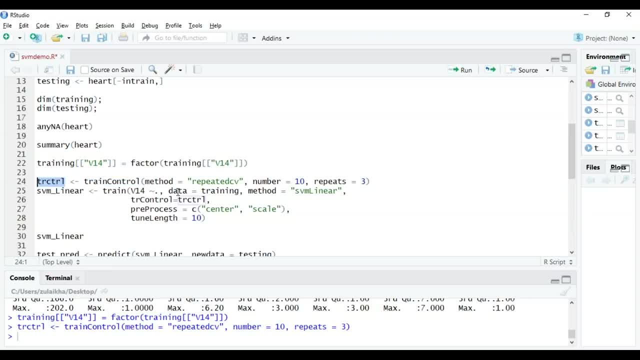 train control method was stored in this variable. okay, so we're going to pass that variable over here. next is the pre-processing parameter. this is for pre-processing our training data set. all right, and these two- center and scale- help for centering and scaling the data. okay, then we also. 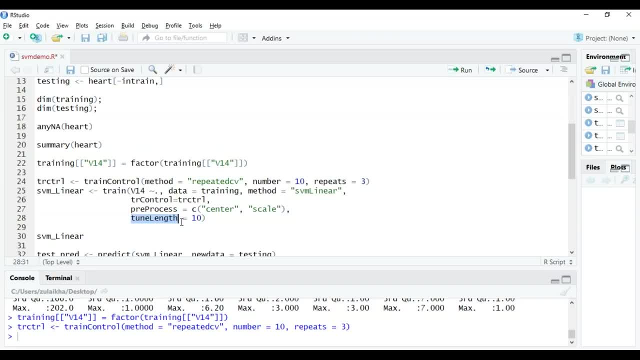 have the tune length parameter. this parameter holds an integer value. okay, this is for tuning our algorithm, so let's run this block of code. all right, now you can see that our model is using all the attributes in our classifier. check the result of our train method. okay, it's stored in this variable, so let's run this variable. 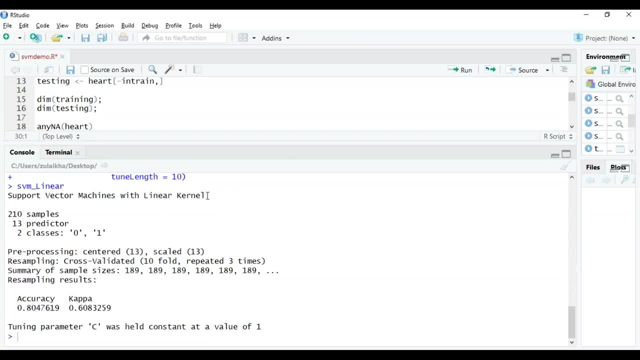 okay, so it says support vector machine with linear kernel. this means that our data was linearly separable and that's why we use the linear kernel over here. now, here is just showing us the pre-processing results, resampling results and our sample sizes. all right, and here c value. 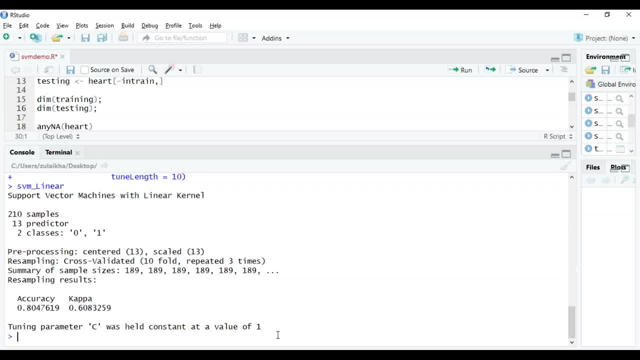 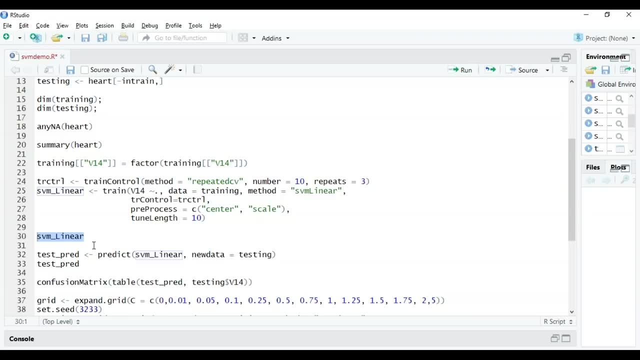 was held at one, because this is a linearly separable model. now, since our model is trained with c value as one, we are ready to predict classes for our test set. okay, we can use the predict method. this is the predict method. now, this method is provided by the carrot package itself. 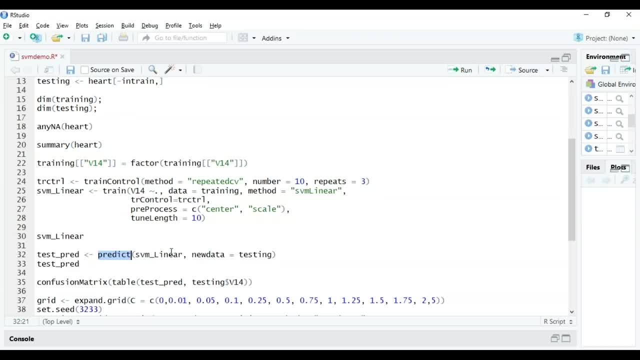 and we are going to pass two arguments to this method. the first parameter is our trained model- okay, what we just trained, spm, linear- we're going to pass that. and the second parameter, which is new data. it basically holds our testing data frame. we created this testing variable at the beginning of a session. 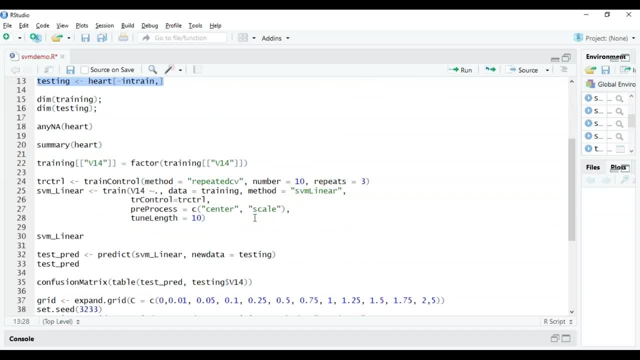 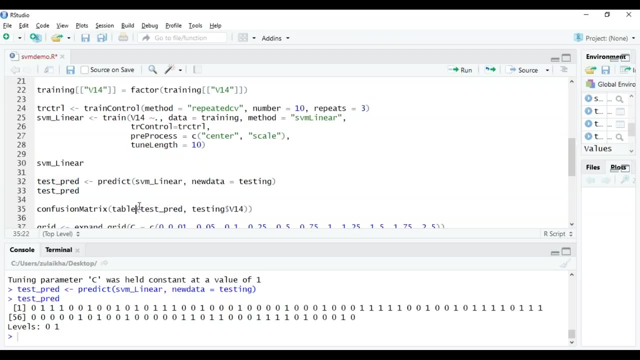 okay, here is the testing variable. we created it to store our testing data. all right, so we're basically going to pass the testing data frame and our trained model. okay, so let's run this. all right, it's run successfully. so if i run our testing model, this one, you get the prediction. 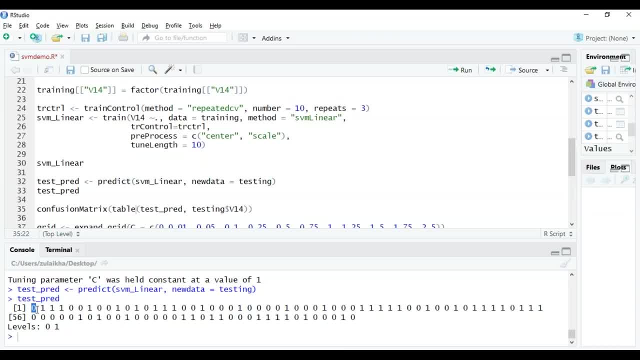 values. okay, so zero stands for patients who have nothing to do with a heart attack, and one is basically patients suffering from heart diseases. okay, so it's showing this for each and every patient. so the zero value represents the first patient, the one value represents the second, one, third, one. 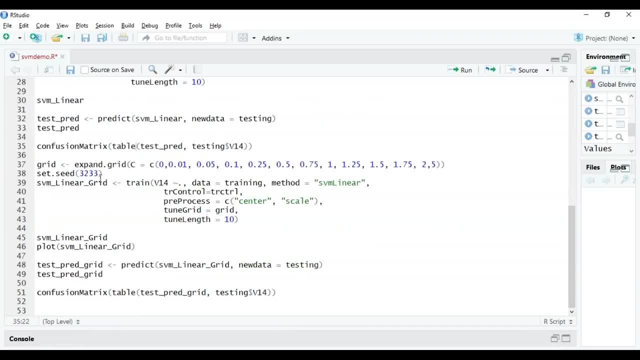 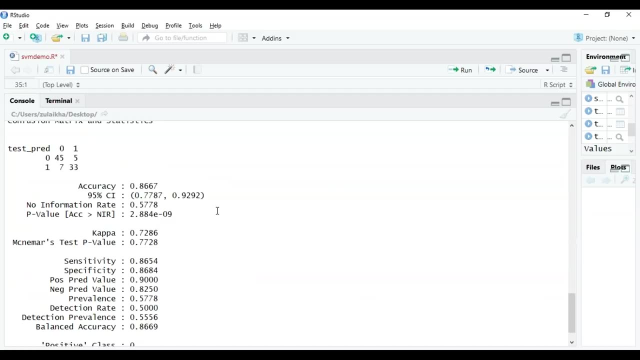 fourth one, and so on. okay, so, guys, this was our prediction. now let's also test the accuracy of our model. okay, we're going to use the confusion matrix to predict the accuracy. all right, let's run this line of code. okay, the output shows that our model's accuracy for test set is 86.67. okay, basically, 0.866. 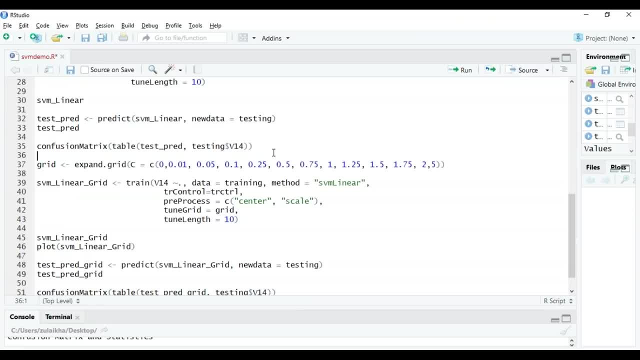 stands for 86.67. now, in order to improve the performance of our model, we can customize the cost value in our linear classification. okay, so in order to do this, you're just going to input values into grid search. okay, this is our grid variable and we're going to input values for c. 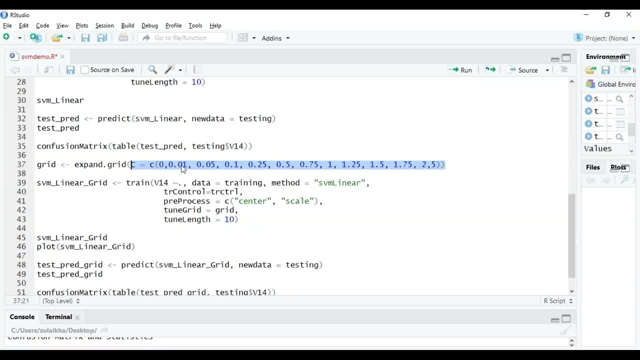 in order to improve the performance of our model. okay, so we're going to put some c values using the expand or grid method, and our next step is to use this data frame for testing our class ifier at specific values of c. okay, so we've assigned some specific values of c, all right? 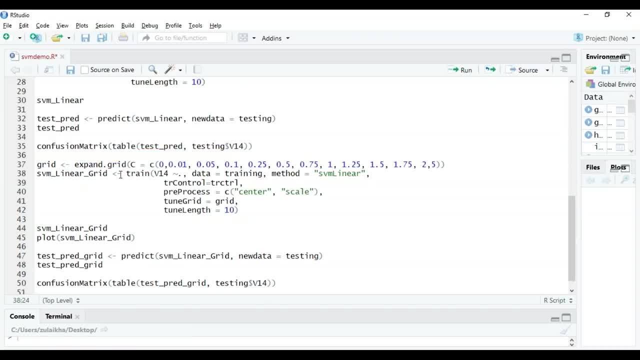 so let's just run this line of code. now we're again training our model using these c values, all right, so let's run this. so, guys, the explanation to this was already told before, so this is the same line of code that we ran earlier. now, if you want to view the model, just 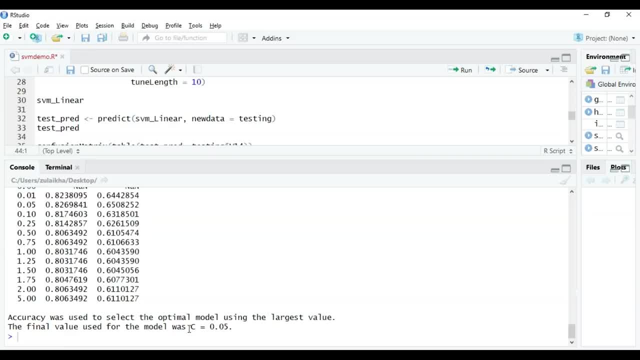 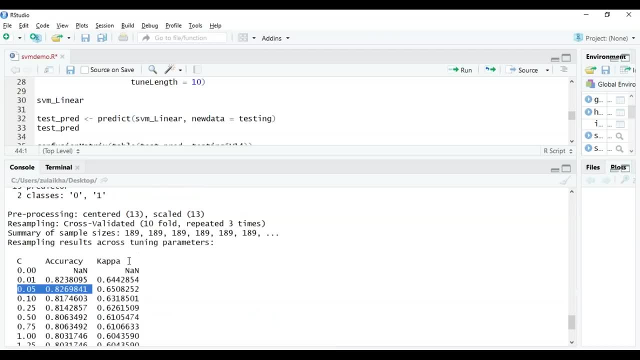 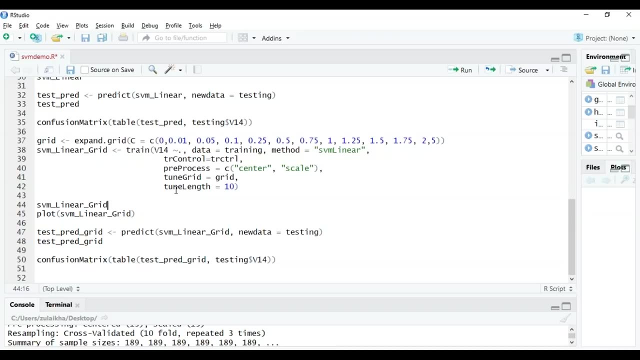 run this line, all right. so now it's saying that for c value as 0.05 accuracy was the most okay. so this is where it's showing the accuracy. all right, so 0.82. so, guys, 0.82 or 82 is quite accurate, because we're not actually feeding a lot of data into the svm classifier. 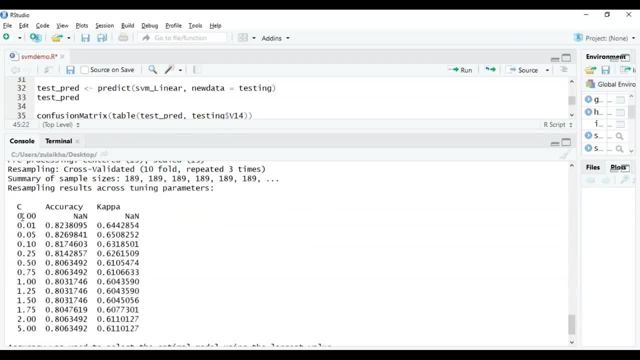 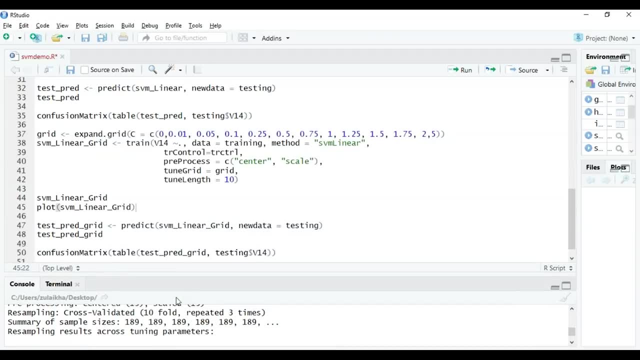 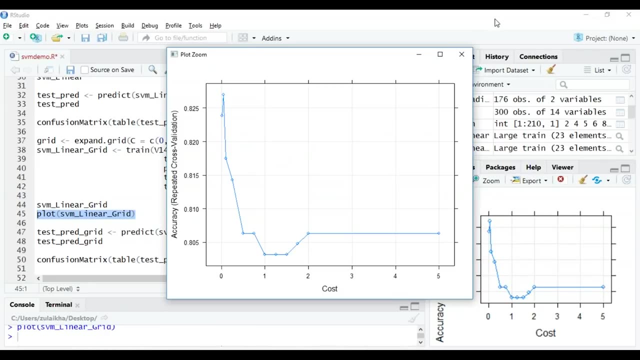 okay, so this basically returns the accuracy level for each value of c. okay, for all the values of c, it's going to return an accuracy level over here. okay, now you can also plot this and try to summarize it, if you want. so let's run this plot. all right, so you can see that for around 0.4 or 0.5, i'm not sure- the 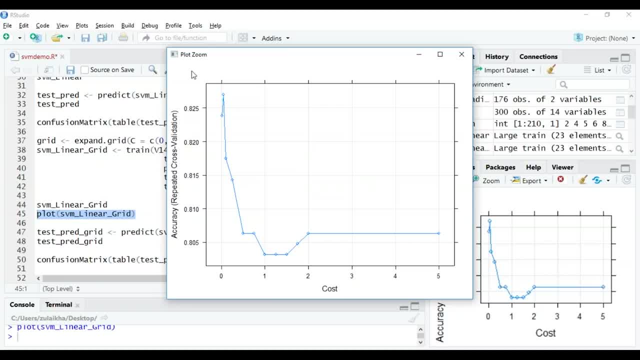 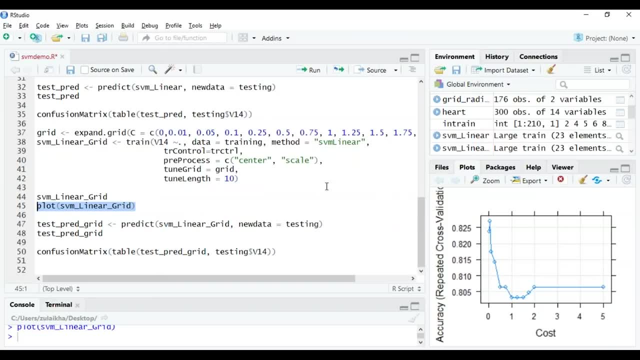 accuracy is the maximum. okay, this is the cost value and this is the accuracy value. all right, so now you know for what value of c you'll have to build your model. so, guys, this was a very easy way to test the accuracy of the model and to check for which value of c our model is the most. 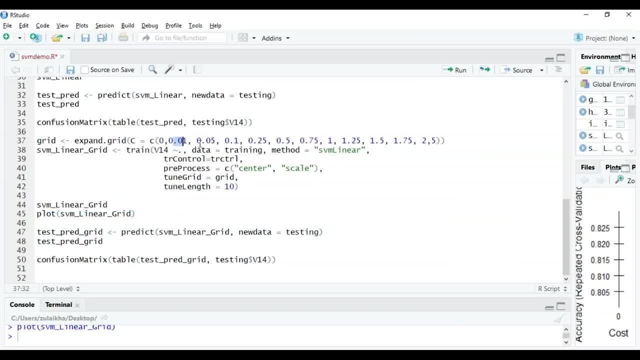 accurate. so now we finished training our model with these c values. now let's test the model for the same c values. okay, if you want, you can do this. so i'm running the same lines of code that i ran earlier. okay, so to the predict function. i'm. 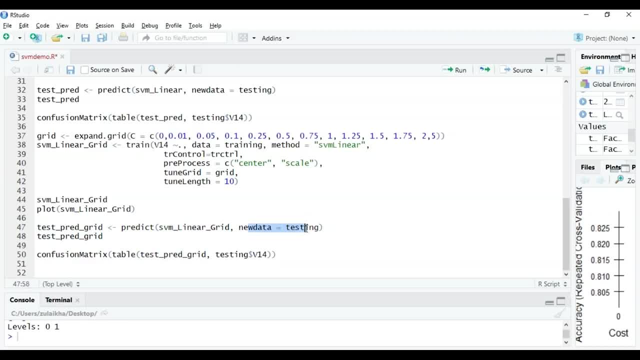 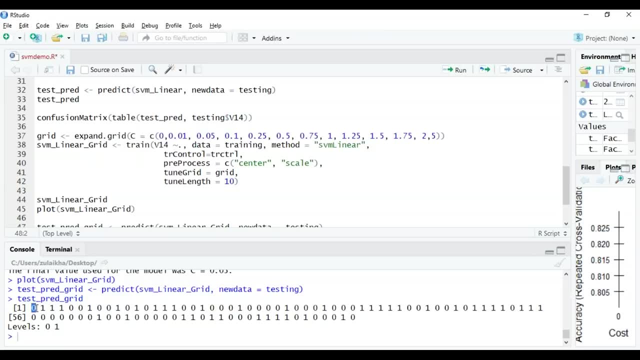 basically passing our training model and the testing data set. okay, then i'm just showing you the output of our testing model. all right, so zero basically shows that a patient is not suffering from heart disease, and one and one shows that a patient is suffering from heart disease. all right, 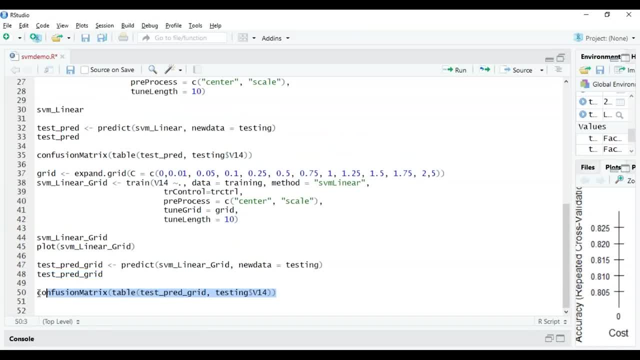 so these were the predictions that we made. you can also again go and check the accuracy. since we created a new testing model over here with different c values, we can also check the accuracy of this model. okay, so i'm passing the name of this model over here and i'm testing our accuracy of. 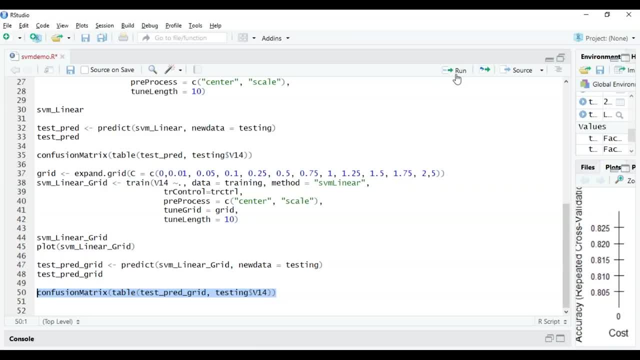 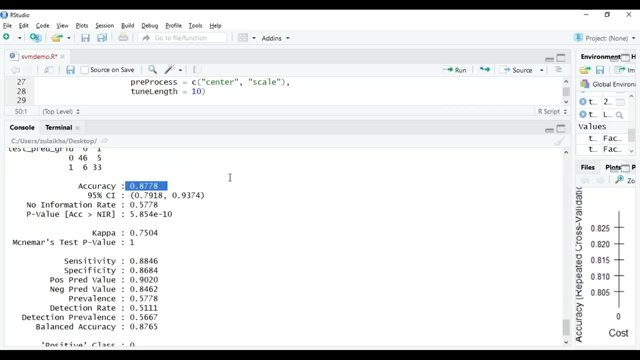 the prediction variable v14. all right, let's run this confusion matrix and hopefully this gives us a higher accuracy rate. okay, it actually gives us a higher accuracy rate. earlier we got 0.86 something. now it is 87 percent- 0.8778- okay, which is obviously more than 0.86. 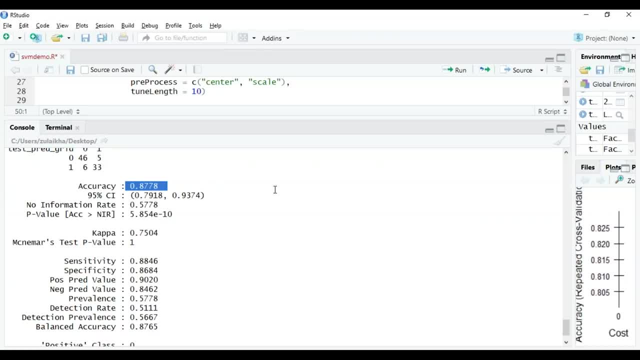 so, guys, this is how you improve the accuracy of your matrix: you tune and play around with the value of c, and then you find out for which value of c our model will be more accurate. okay, so, guys, this was a simple demonstration of how svm can be used to predict whether a patient 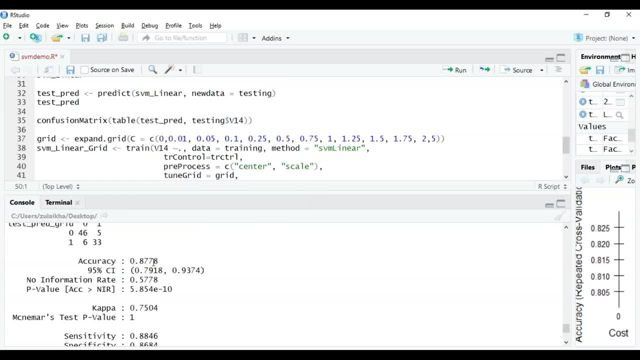 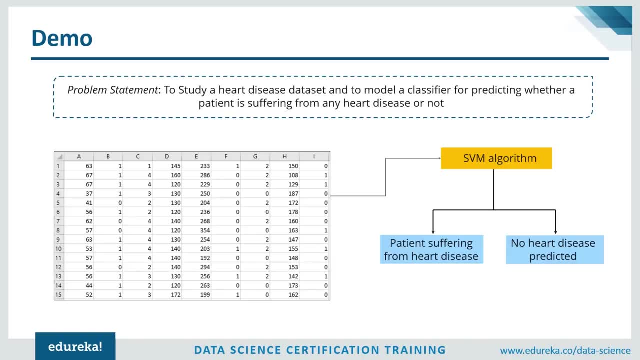 has a heart disease or not. okay, and it was quite good because it was 87% accurate, which is a good enough number, correct, all right. so let me just summarize what we did in the demo, okay, so we basically studied a data set which contained many patients with 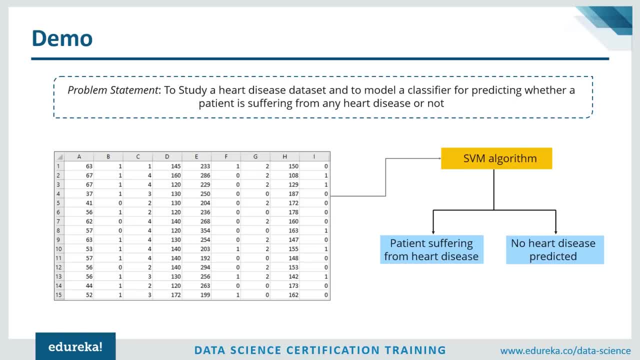 information, such as their age, cholesterol level, their sex and etc. okay, we studied these different attributes of each patient to predict whether a patient will suffer from a heart disease or he will not, and we use the linear svm algorithm to do this. okay, and in the end, we build a model with an. 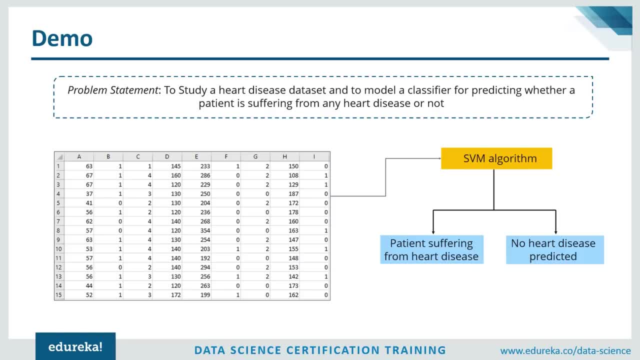 accuracy of 87% accurate, which is a good enough number, correct, all right. so let me just summarize what we did in the demo. okay, so we basically studied a data set which contained many patients with information such as their age, cholesterol level- 87.78 accuracy rate, which is pretty good. so, guys, 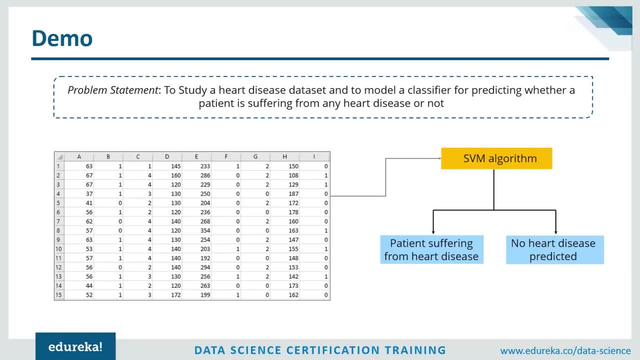 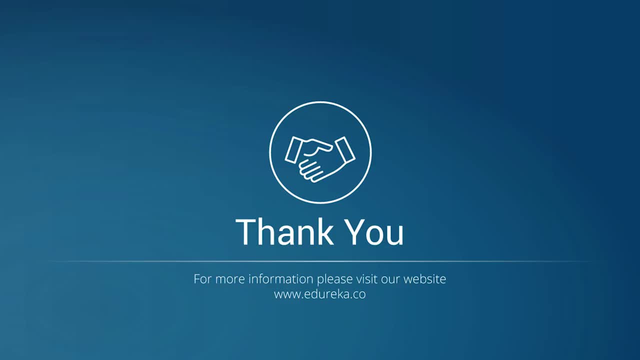 give yourself a pat on the back, because now you've successfully run a demo which shows how svm is a very accurate classifier. 87 is pretty good. so, guys, with this we come to the end of today's session. if you have any doubts or queries regarding our session today, please leave them in the